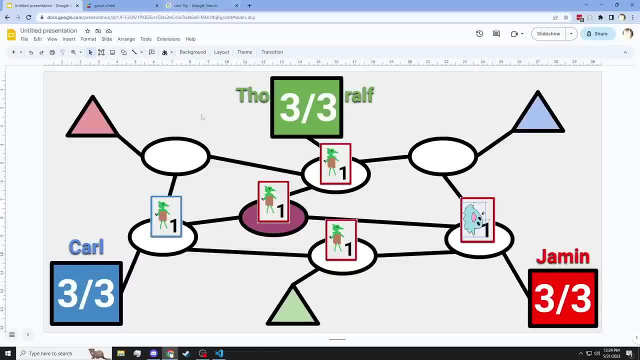 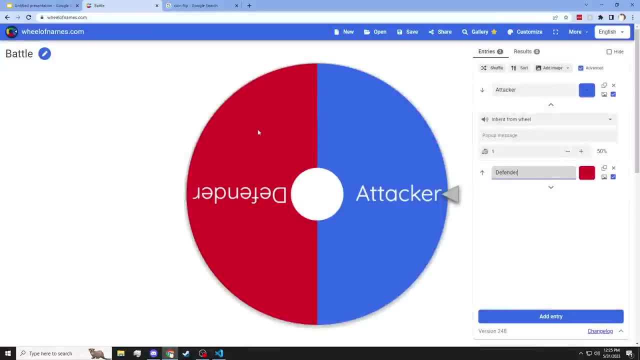 This is going to be. He's so short Tails, I'll move my bottom goblin one to the left That will fight with Carl's goblin. Indeed, If you win this, you're the only one with goblins. 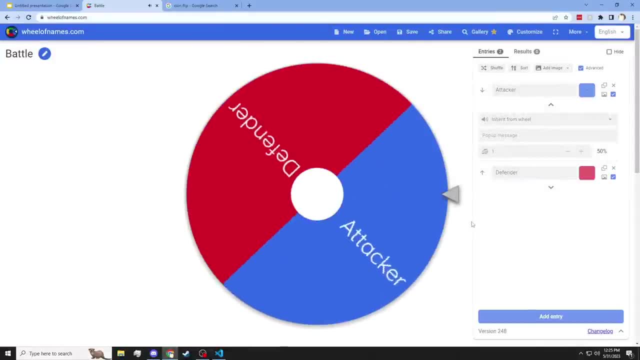 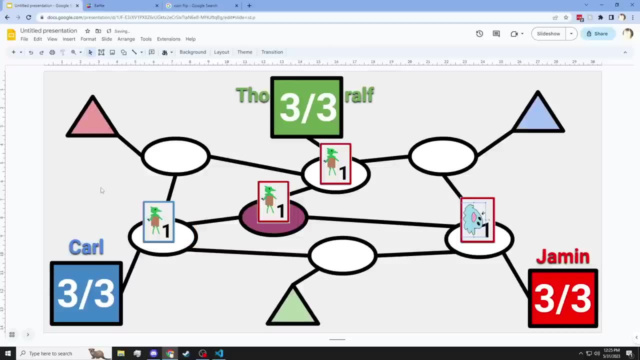 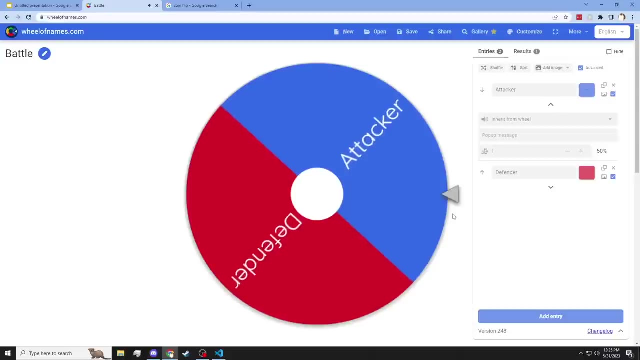 Or any creatures. Oh wow, Yay, Taking down the Monopoly. I'll move my middle goblin towards Carl's goblin. Oh no, the slime is going to farm the good wheel. The attacker will win, Alright. and then my top goblin moves into the middle. 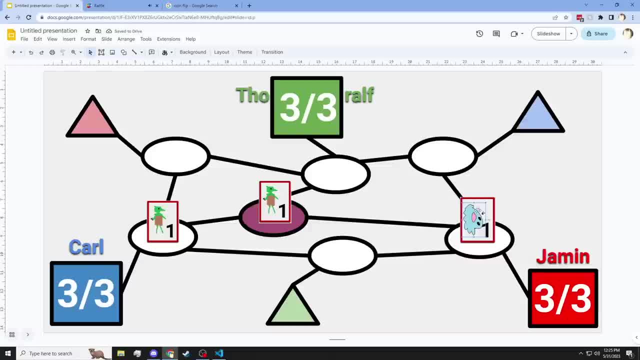 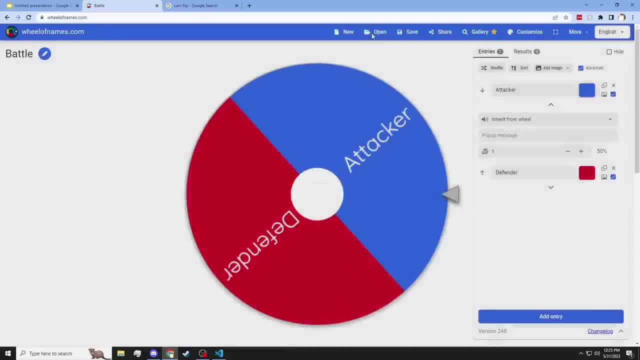 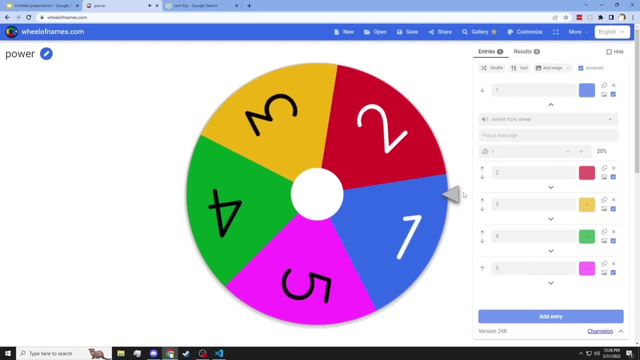 Into the middle. Jamin's too good at this game. And then my slime moves to the left, Carl, it is now your turn. Please win Heads. You now make a creature. No, No, You can beat all of the other creatures. 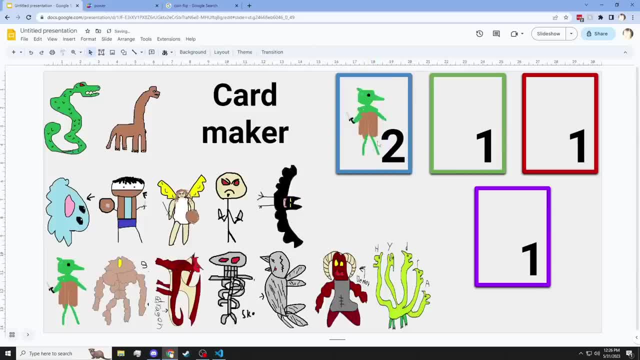 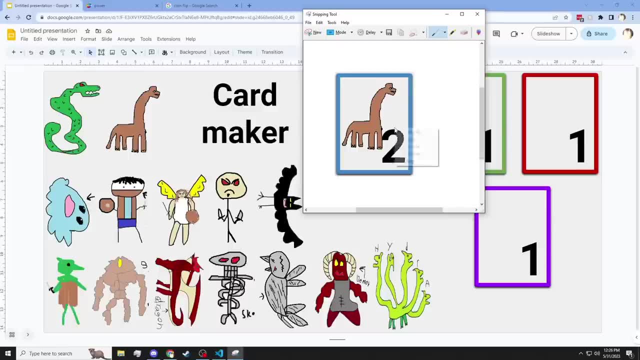 Is it going to really confuse you if I pick the goblin? Nah, Oh, no, Wait, can I pick the yamen? Oh, that's it. Yes, I love that you knew. Why are there four colors. Don't worry about it. 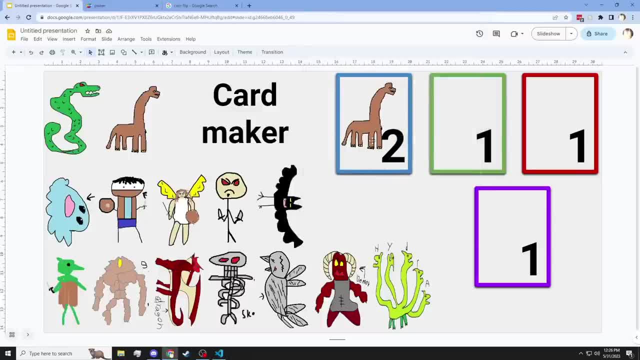 Hmm, Are you joining the game? I'm not. I don't see where there's a fourth color right now. It's your turn, Carl, It's chomping time. Would you like to reveal your card's ability? Yes, 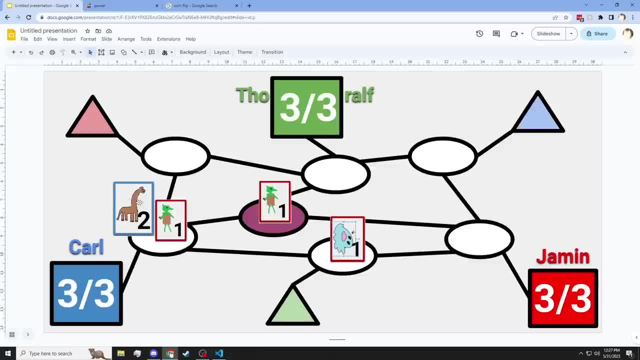 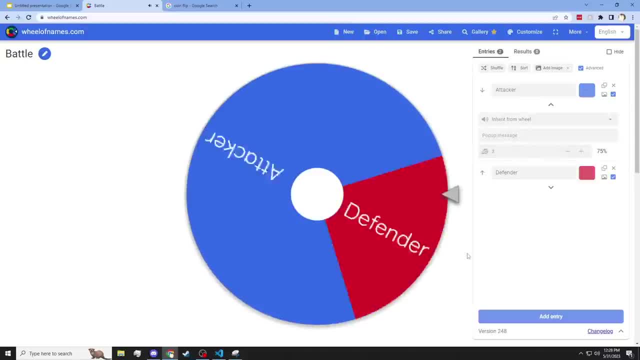 If this card battles another card with less power, this card gains one power. It is now a three power dino. It also becomes bigger. That's cool, Okay, Oh Easy, I win those every time, See, No What. 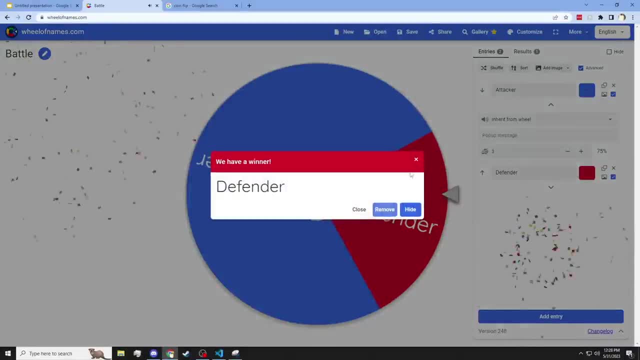 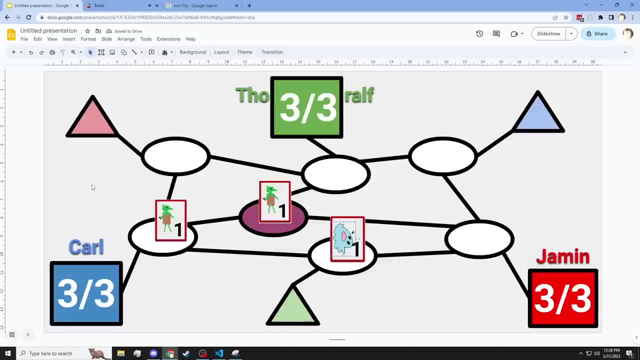 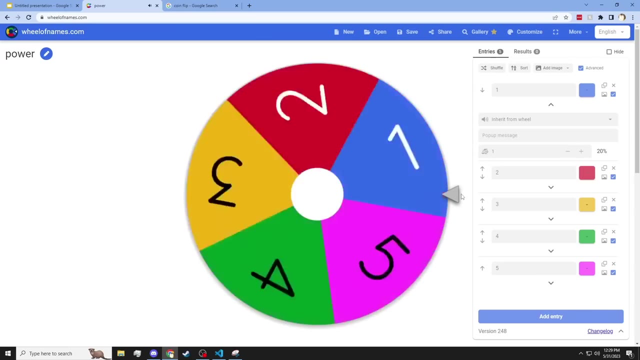 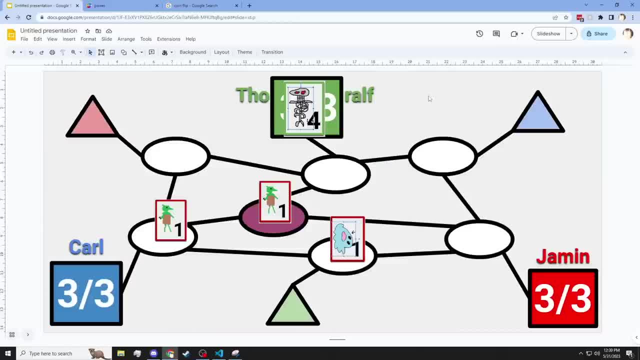 Heads, Heads, Heads, Heads, Heads, Heads, Heads. Wow, I'll take it. I'll take the skeleton If it's an end of the battlefield ability, can I just say it? Yep, When this card enters the battlefield, it gains control of a goblin. 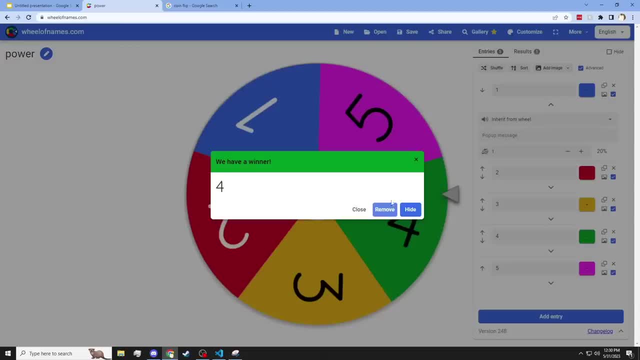 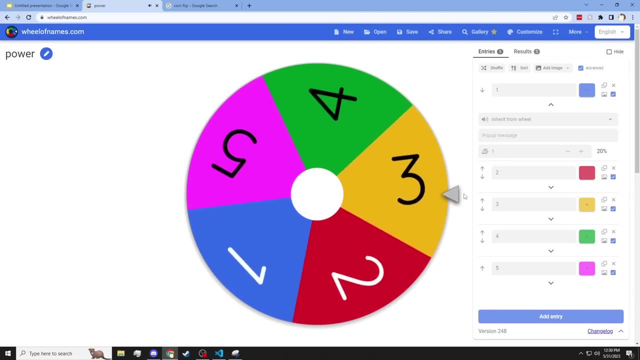 You have the goblin in the middle. I would like my four. one step ahead. Jamin, you're up Heads, you make a new card. Heads, Heads, Heads, Heads, Heads. One, One, One One. 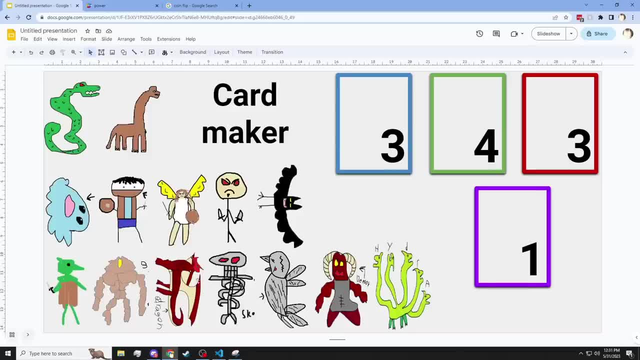 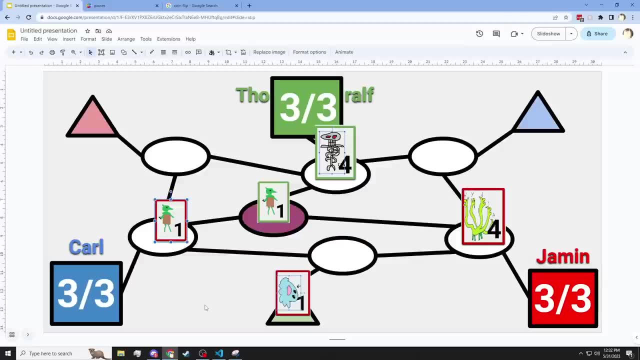 One, One, Alright, alright. Three power. I'll have the hydra, please. You now have a four power, hydra. Yeah, That one will move up one space. Yeah, the slime will move down onto the triangle. Oh, that's also mine. 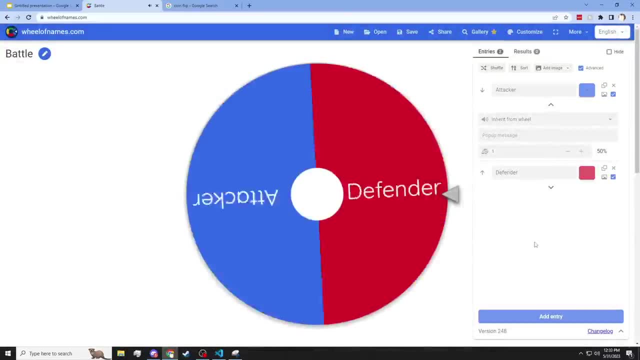 Of course I'm gonna fight Toffle, I'm winning. Called it No. No, I'm doing the Jamin strat. Okay, Scar, It's called the Jamin strat, not tienes Sábado strategy, for one reason: 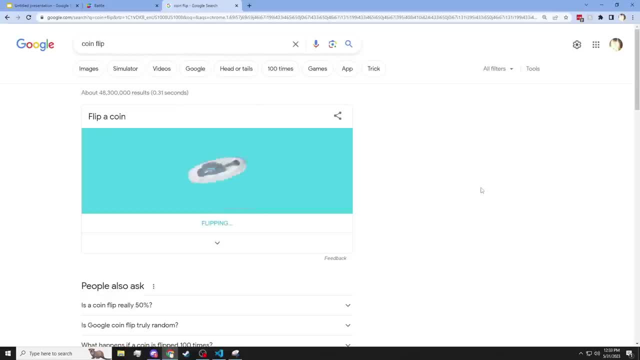 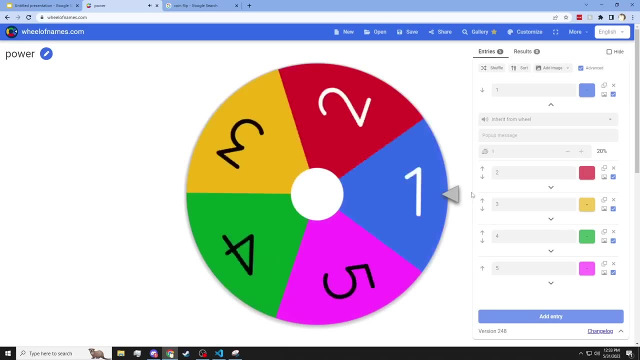 Attacker wins. Karl, you're up If I don't make anything. I'm just on spectator mode, right, Pretty much. Hey, you get to make something, I'll do the yamen, It's a five. Oh no, when he said it's a five, he got a one. 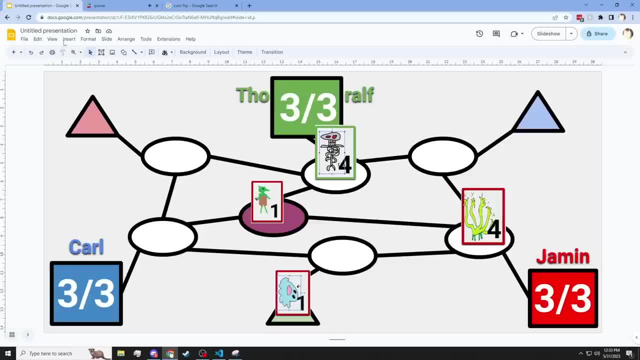 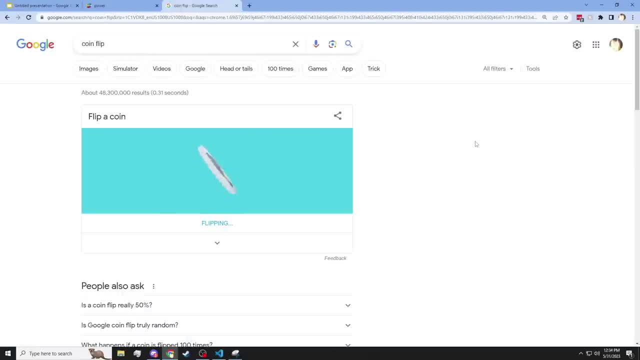 I did do a yamen. Um, I want the guy with the shield, but a comically small butter knife Toffle. you're up Tails Alright, walk into the middle, Smash the goblin Toffle, you know. 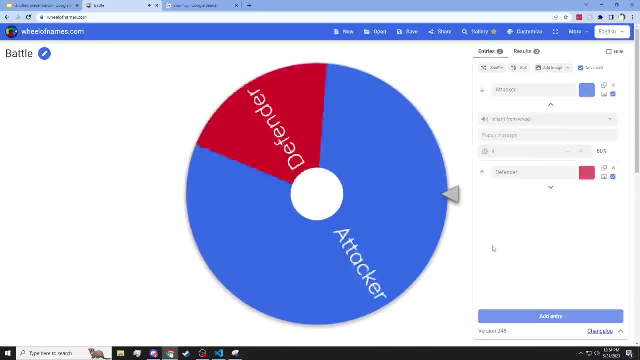 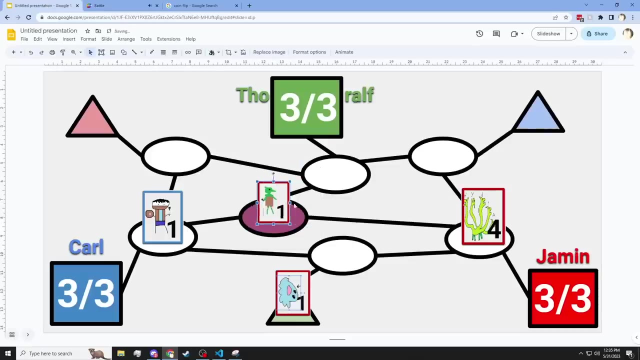 it's not gonna work. It's gonna work. I have full power. Look at the red square. Look at the board. Would you please look at the board? Toffle, Toffle. That's unfortunate, Jamin, you're up. 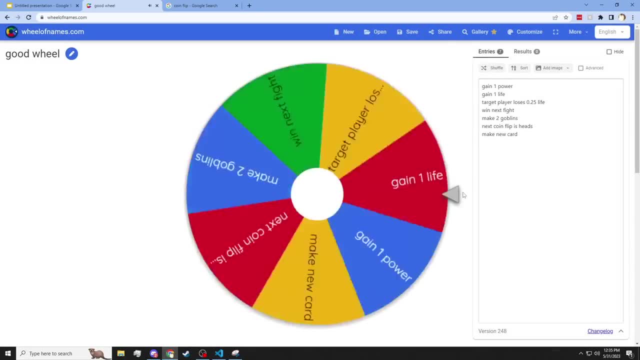 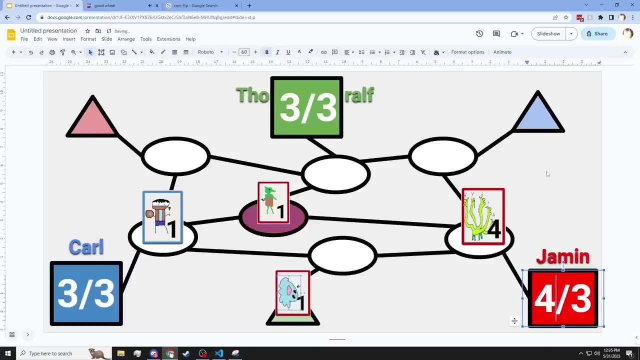 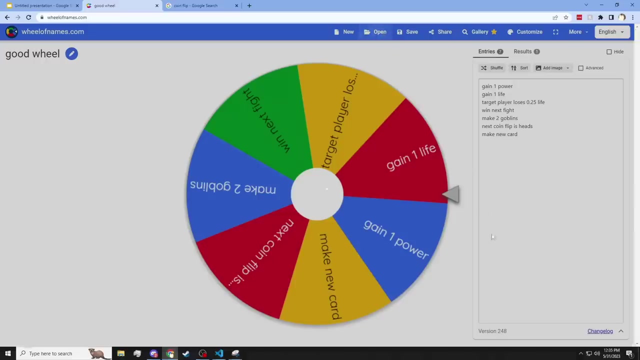 You get to spin the good wheel. Nice, Oh, that's convenient. Alright, I'll take it. Wow, You're unkillable. now Let's see. if you make another creature Heads, you make another creature. Jamin is really good at this game. 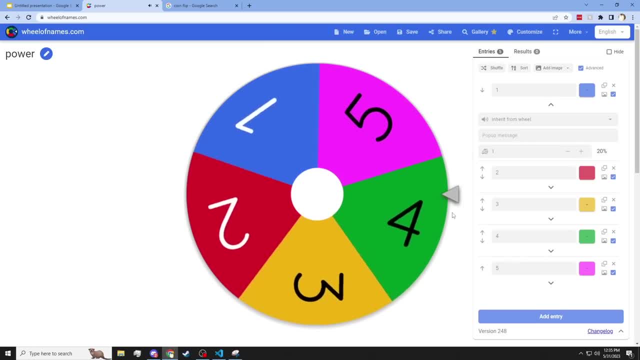 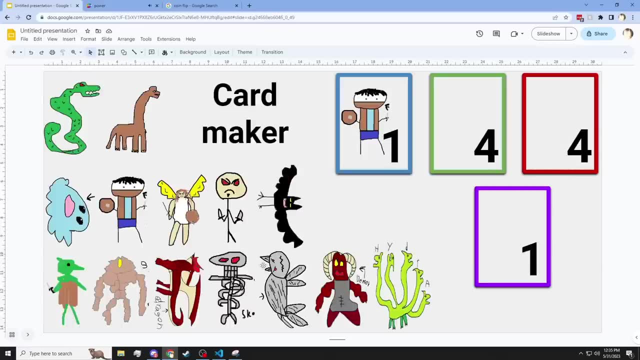 I am. Come on five. No, no, You are very good at this game. Full power. What will it look like? It'll be the buff golem with the yellow eye. Oh, I thought it was poop. You thought it was poop. 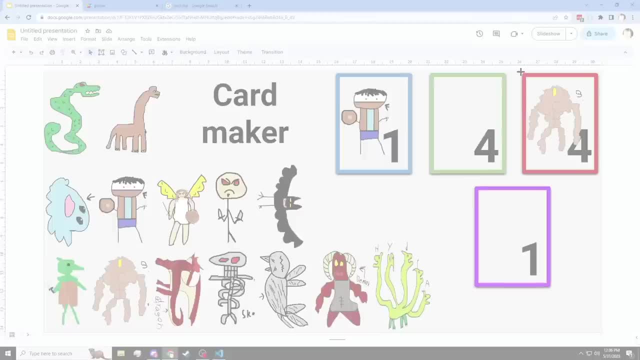 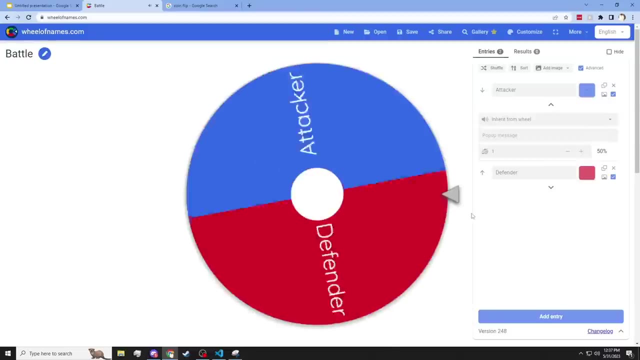 I actually thought that was supposed to be not buff. I thought it was like kind of immature joke. I'll move my goblin onto Carl's bandit. Oh, come on, I have only one, Carl. The game has not gone great for you. 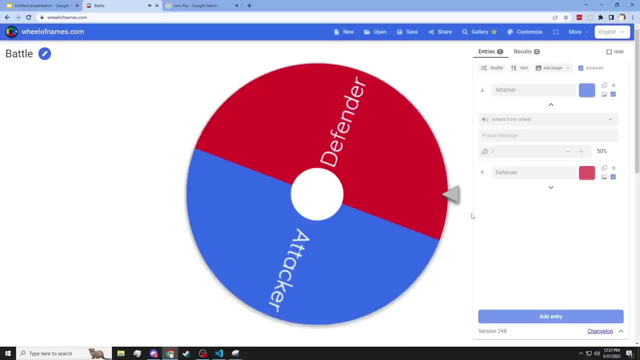 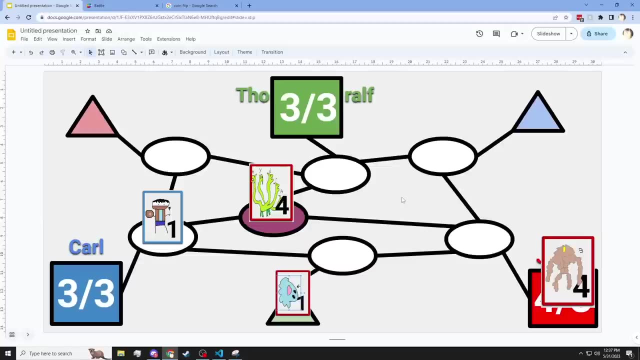 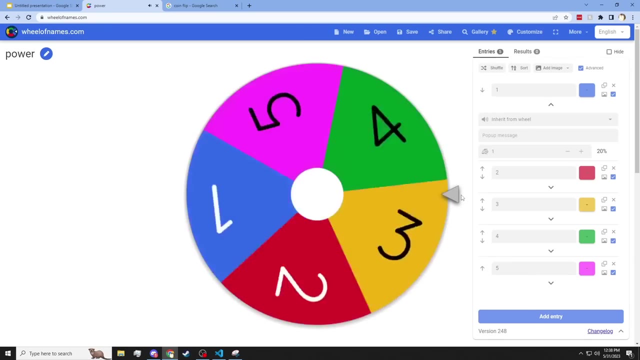 It's really not. Oh, there's a turn of events, Second win. Do you guys think my hot pants guy can take on the Hydra Historically? no, Carl, you're up Heads. Oh right, I have to pick two power. 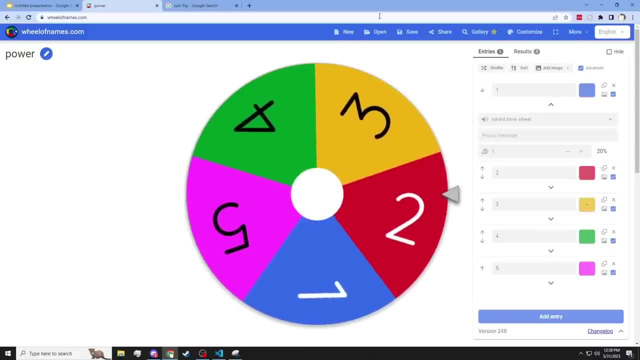 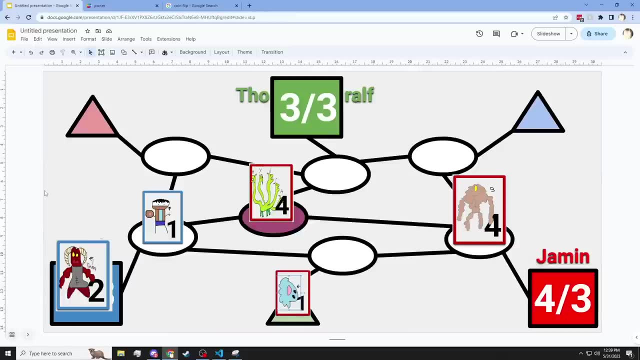 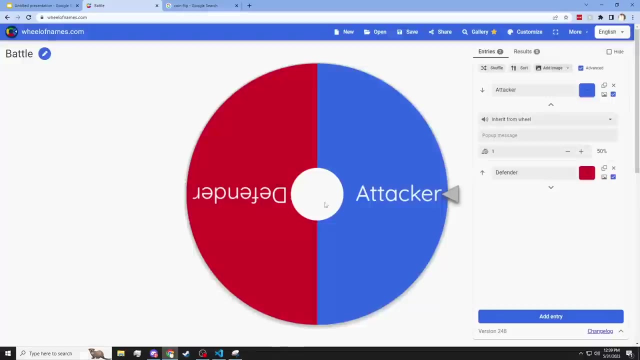 Oh yeah, Okay, that's better than a one. I want the guy with the abs, The demon See. Should I attack the Hydra with my short-legged thief? Let's do it Now. I'm actually afraid This is like a 50-50, actually. 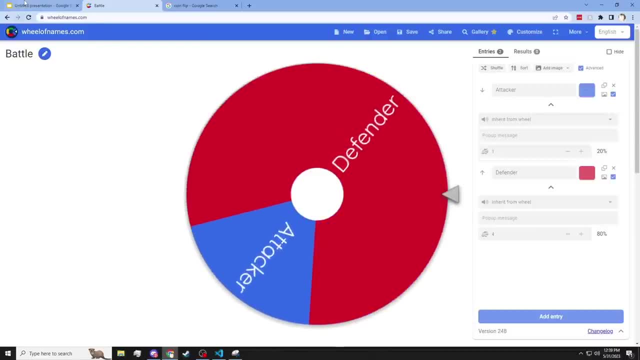 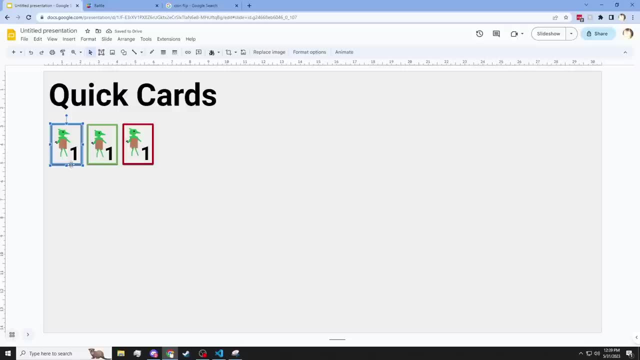 Oh, no Defender is going to win. I do have a trigger, though. When he dies, I make a goblin. Why do you make the goblin? I'm throwing another one at it. Does the goblin have any ability? 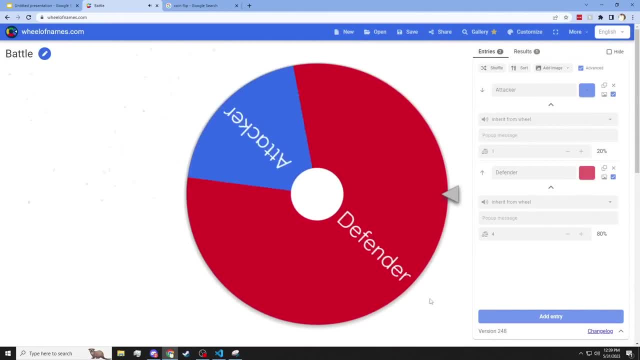 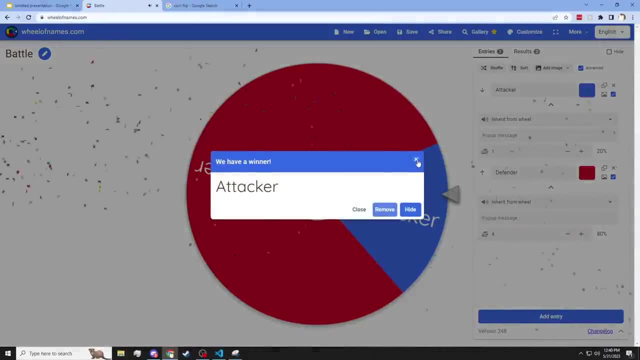 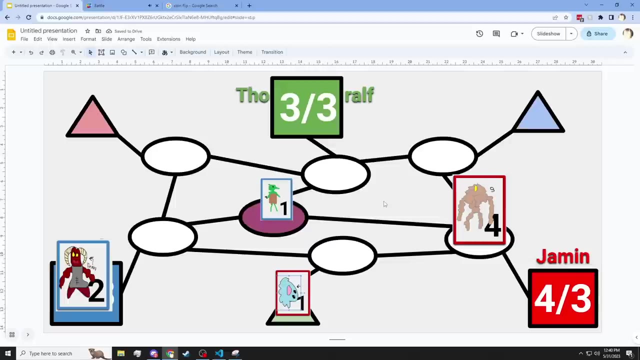 It goes down to 25% of winning. That's how coin flips work. Oh, Ah, No, Yes, Yes, Hit it. See, That's how coin flips work. Okay, My first time on the goodwill- Not yet. 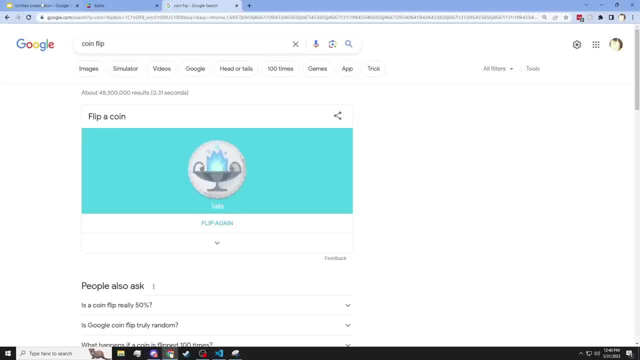 Toffle, you're up. I don't make anything. Toffle has no turn. Jamin, you're up. Um, yes, Let's create a creature. Nope, Please don't kill my goblin. I kind of have to, Carl. 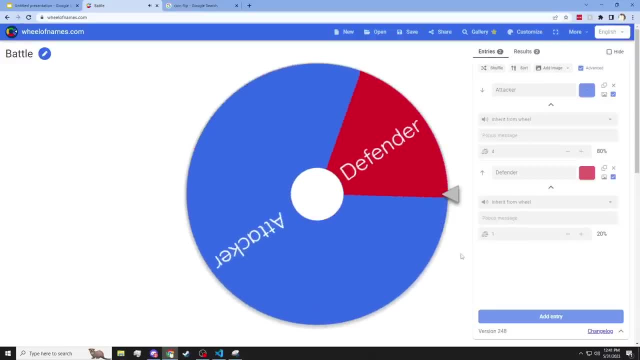 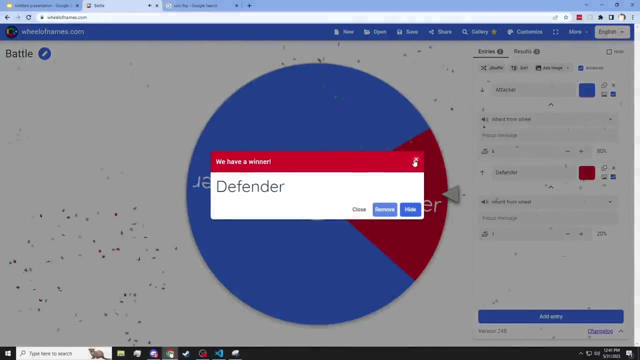 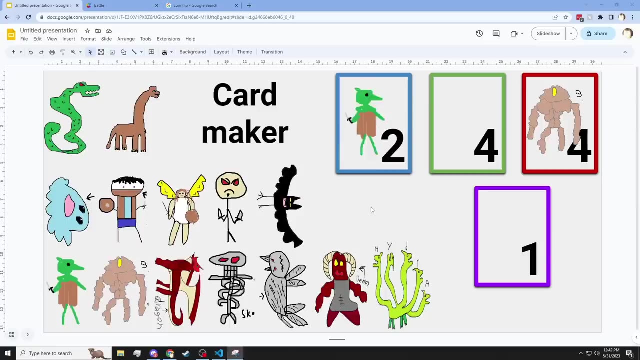 Golem versus the goblin. Oh no, No Goblin. Can I have an extra power on my goblin because it's defeated two legendary creatures? It's upgraded level. I think You know what. You're probably right. It has defeated two legendary creatures. 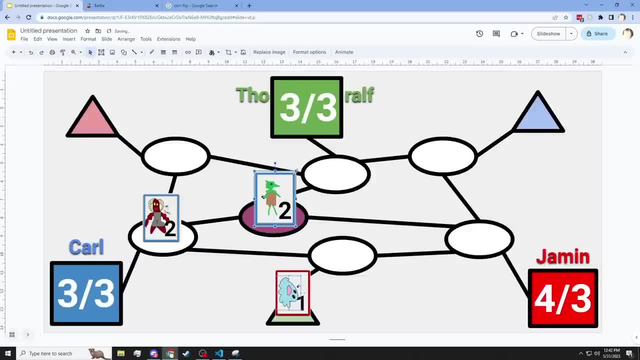 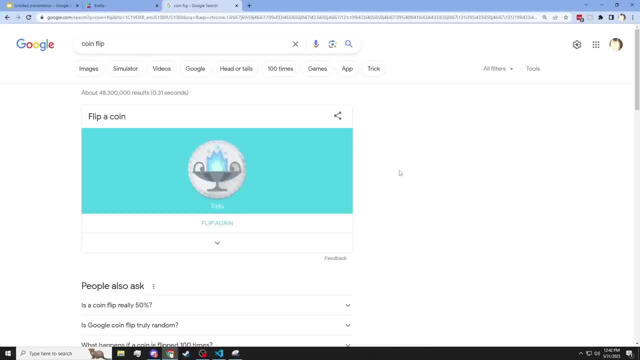 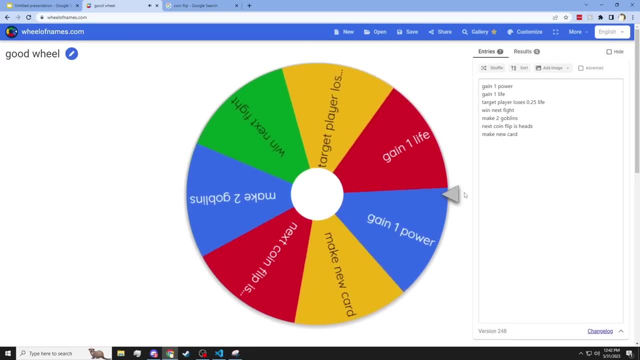 Remember when I had all these creatures in the center square and stuff. Now you just have a towel on a triangle. that's not even yours. Carl, you're up, Oh, after all this. Yeah, Make two goblins, Make two goblins. 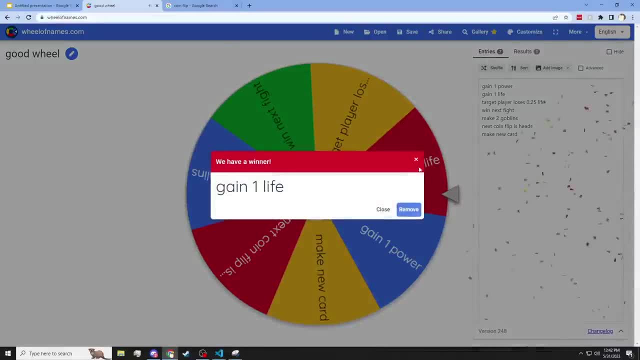 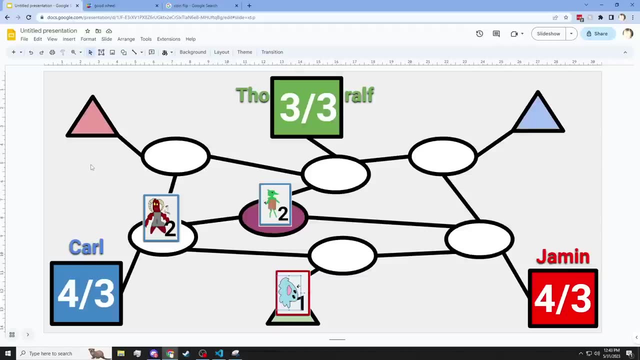 Ah, that's okay, You gain one life. I really like the bueno wheel, but I also think it's time to try to take someone down. Guys, I need your arguments. Who am I rushing? I win. Do you have a counterpoint? 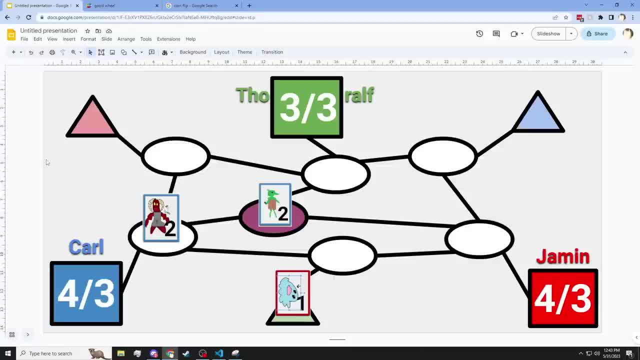 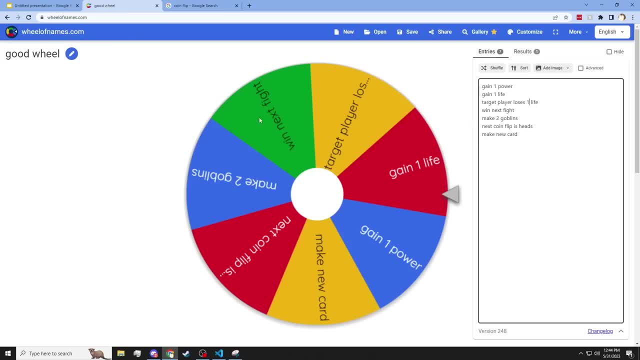 We both have four life. Carl, Are you trying to get on the same level? like we're friends, I see a bit of myself in you. We're in the same tribe, Toffle. you're up Heads, So no matter which creature. 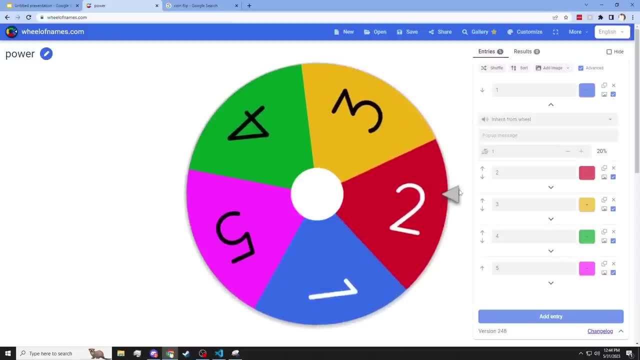 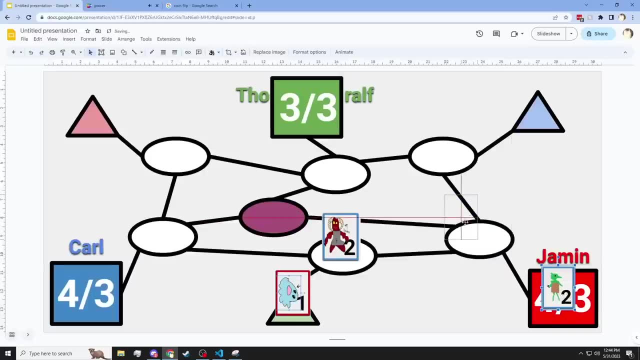 dies on an opposing square, it deals 0.5 damage. Was that it? No? when a creature gets to, let's say if this creature would die, Carl would make a new goblin and you'd lose one health, I see. 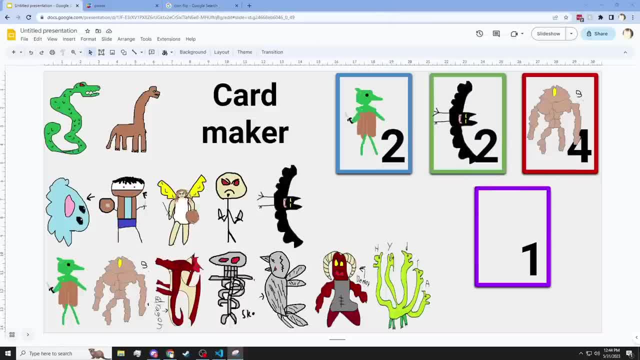 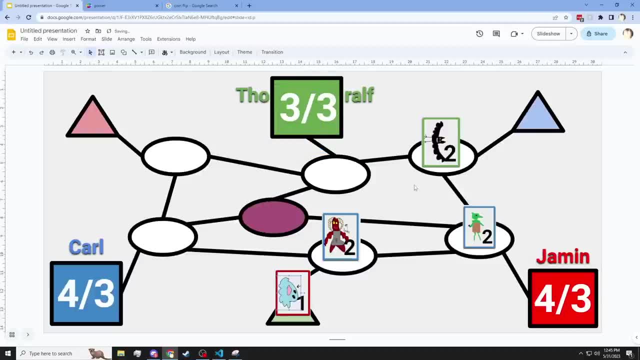 It's not too strong, So we'll take a bat. So my assumption is this bat can fly so I can move to different spaces. Now everyone is just trying to metagame. Oh perfect, I love it. Jamin, you're up. 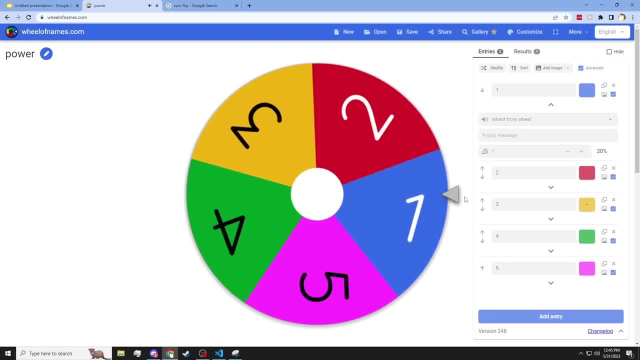 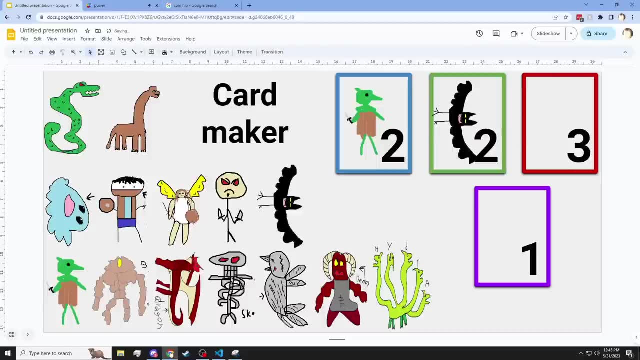 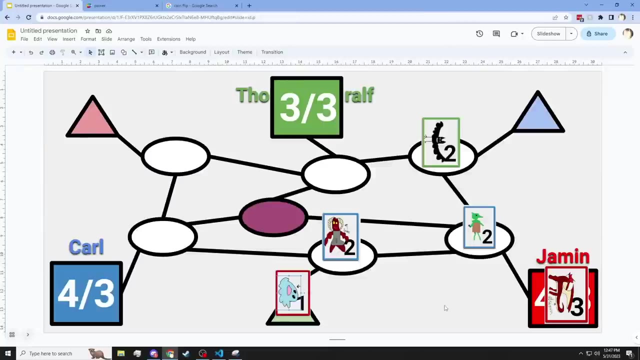 Heads. Oh no, Yeah, I can. Yes, Three, And then I'll pick dragon. Yeah, you wouldn't have known what it was if it wasn't written dragon next to it. Exactly, I'm just that good of an artist. 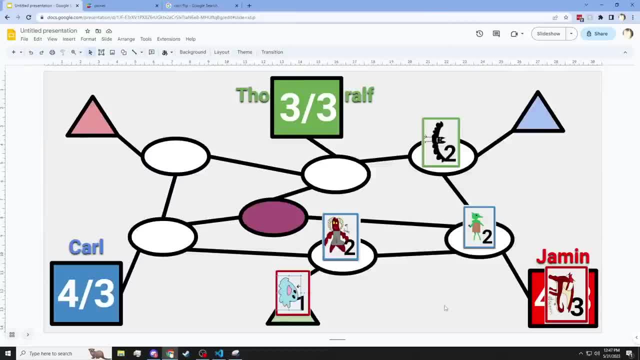 Toffle. could I convince you into a deal where Carl loses his board? What? And you don't have to do anything? How is Taladf involved in here? Okay, all you have to do is So you just have to swear for a bit. 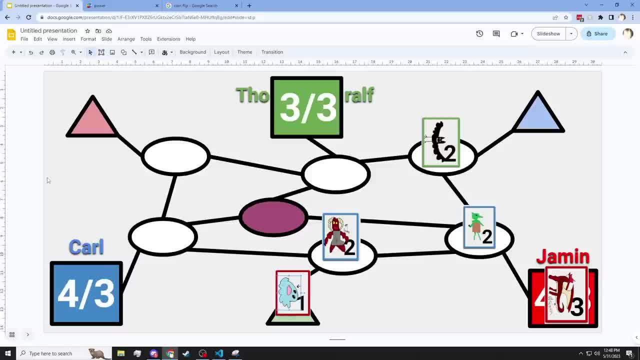 Any swear word. Hi there, this is the editor, Noah, and I'm going to tell you how to swear whenever a player swears. So essentially, what's happening is he's telling Thorof to swear and it will activate the ability a bunch of times. 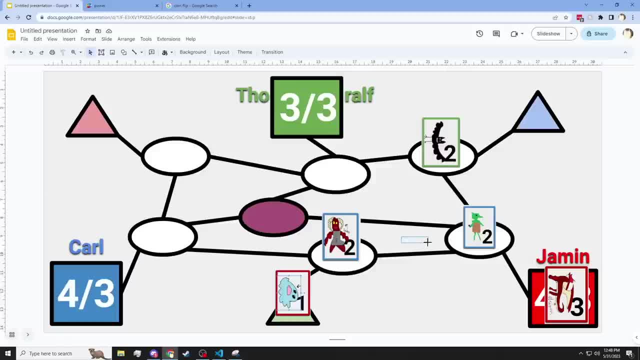 So if you don't hear him swearing, just know that I decided to edit it out, even though all the swearing is done in German. Alright, back to the video. That was like five times right, Probably, So my slime on the bottom has the ability. 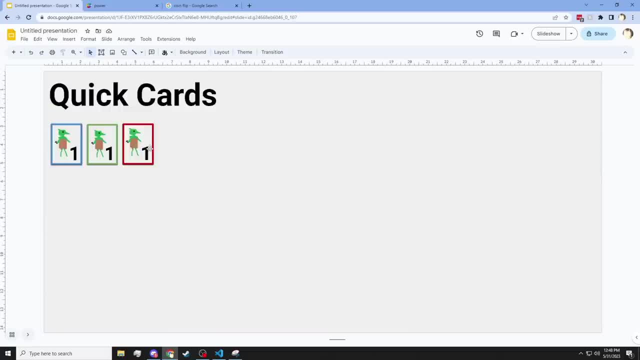 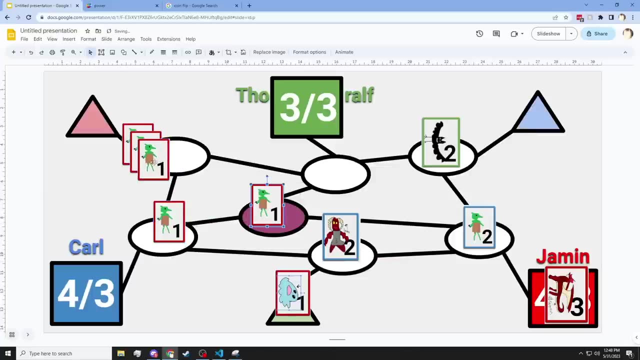 whenever someone swears, I get a 1-1 token. Oh wait, So if you swear five times, you get five 1-1 tokens? I would hope so. So you were just banking your slime on a safe space because you didn't want to. 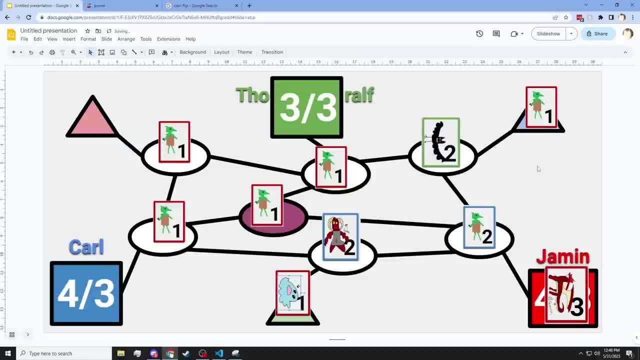 I was wondering why it chills in the corner And my dragon has the ability. whenever someone swears a thing of my choice loses one power. So I will reduce the power of all of Karl's creatures to zero. Wait, they both have the swearing combo. 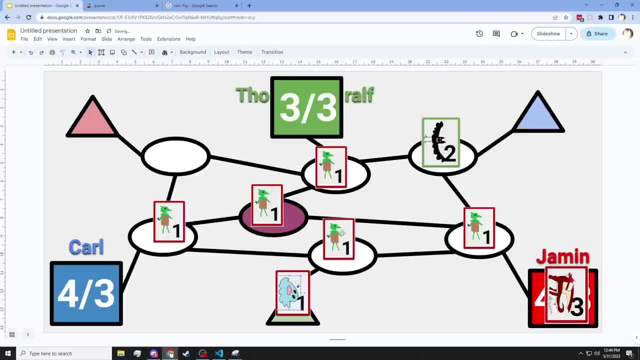 Wait, wait, wait. that doesn't really feel like I didn't. Oh god, I got paid. I got paid. oh no, I don't. I could reduce your card's power one more time, but I won't because you were nice. 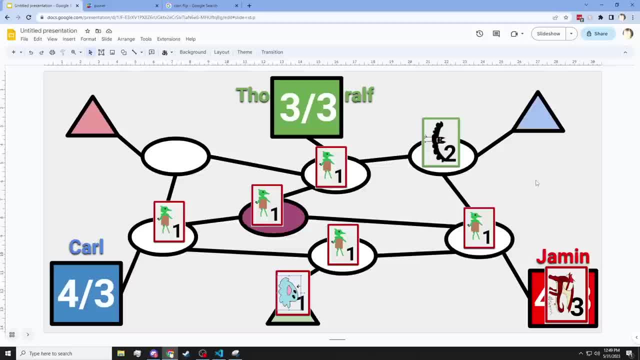 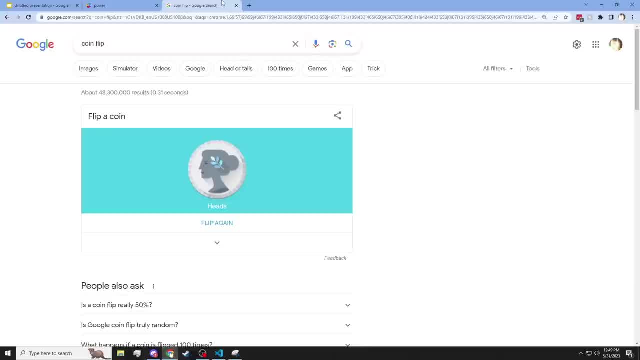 Yay, Okay, Okay. so that was a commanding turn from Jamin Karl, you're up. I better not swear anymore. Yeah, I'd like to make a creature, Nope, Okay, then Toffle, you're up. 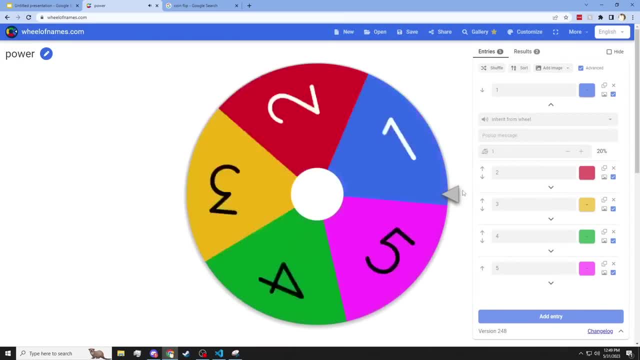 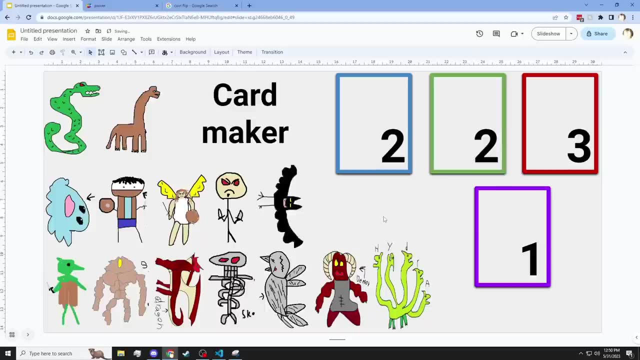 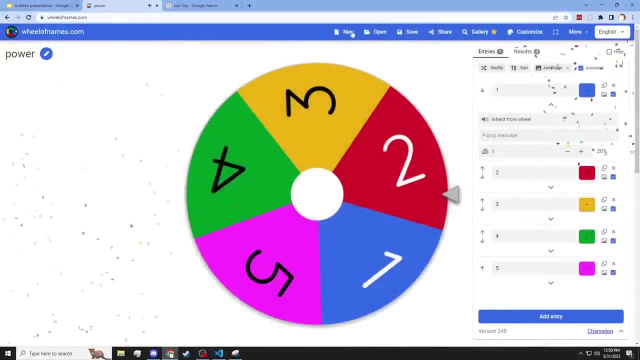 Heads, Heads, Heads, Heads, Heads. All right, Well, we'll make another bet. Then the top bet moves on the goblin. Do you regret some of your words now? Five of them specifically. Look, my mom said I shouldn't swear. 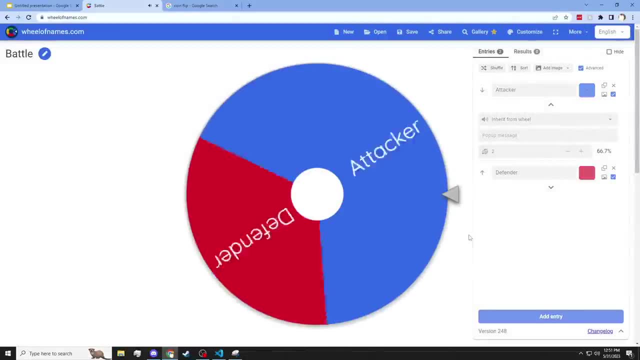 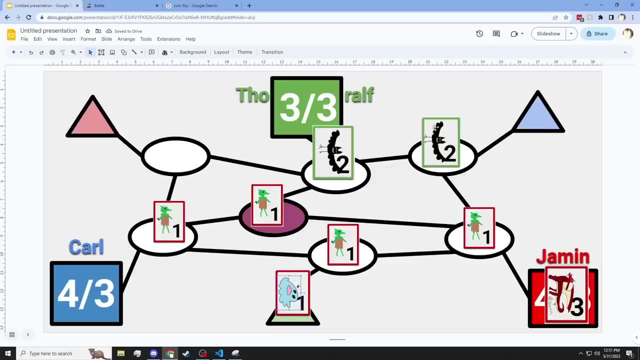 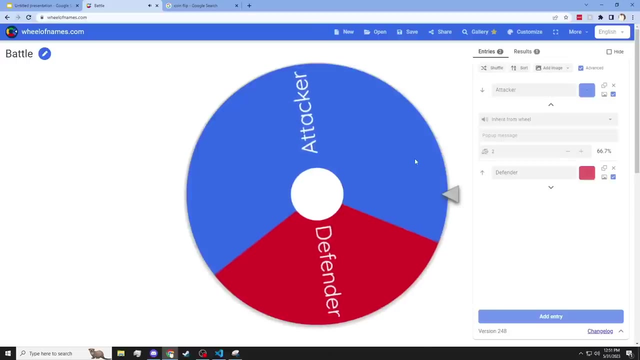 and I didn't believe her, but somehow she was right again. I mean, this red field looks so tiny, Attacker wins Top crow, moves one down to the goblin. Doesn't a flying creature have advantage against a ground creature? Well, it's dead anyways. 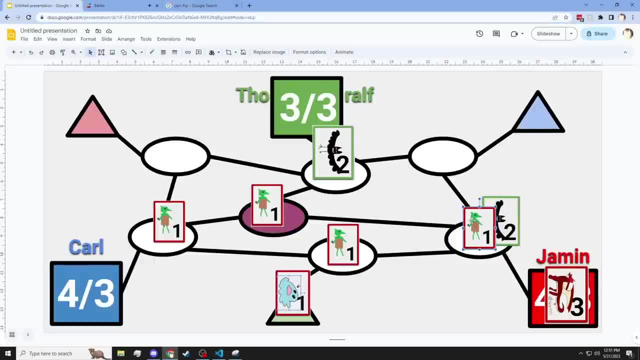 That's why you're winning all your rolls. I like the applause. Thank you, thank you, thank you. They really hate goblins. Jamin, you're up. I mean, I get to spin the good wheel, right, Yep. 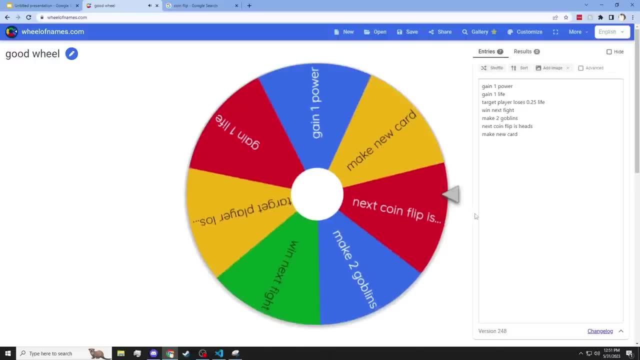 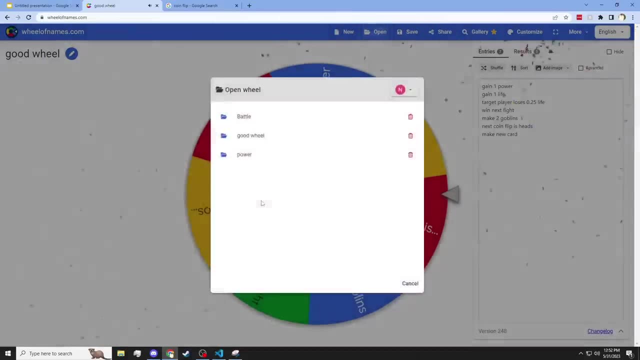 Ooh, Ooh, All right. I mean I guess it's okay. Okay, next coin flip is heads. All right, so you make a creature. now I'd like to specify that the next coin flip is my next coin flip, not the next coin flip. 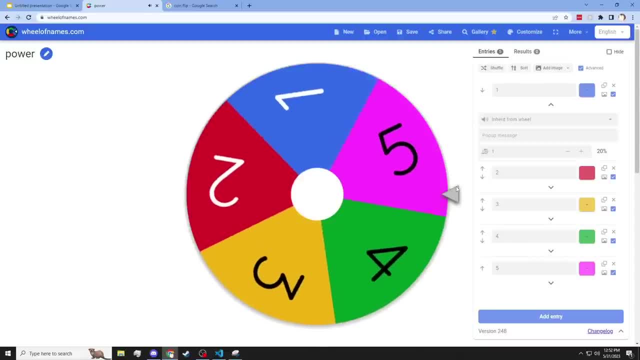 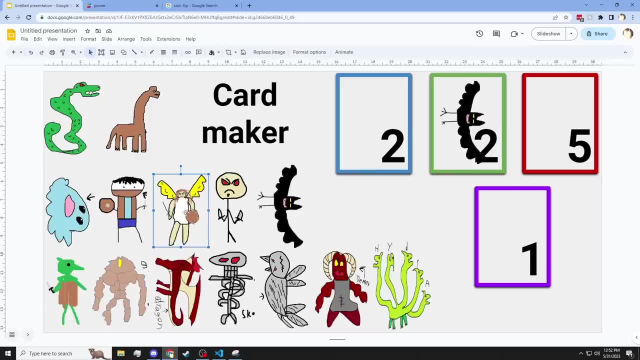 Yeah, you're making a creature. Oh, Oh, I see I'm doing that right now. Wow, Five power. I mean we didn't have an angel yet and it does seem like the strongest thing here, so I guess that kind of pushes my dragon. 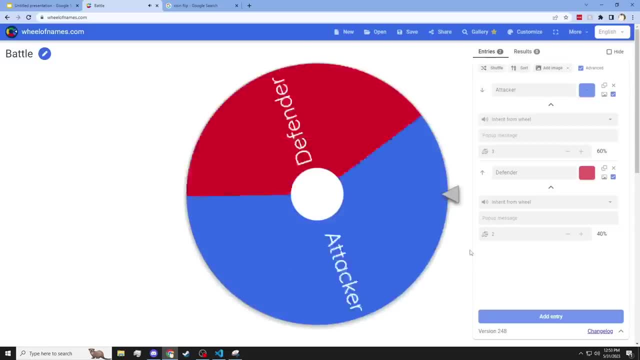 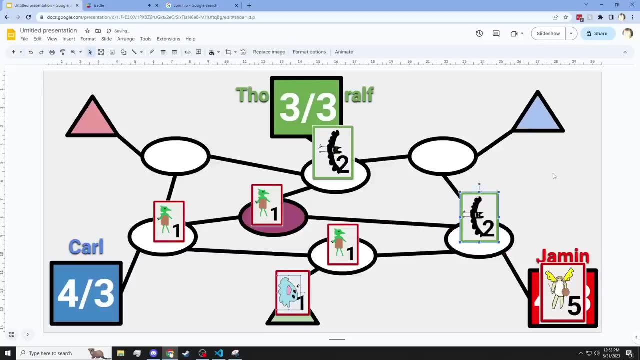 onto the thing. That's unfortunate, Come on. No, It is now 50% better to swear now. Yeah, Anyone want to go for it? No, I guess the left goblin moves up one. The bottom goblin moves left one. 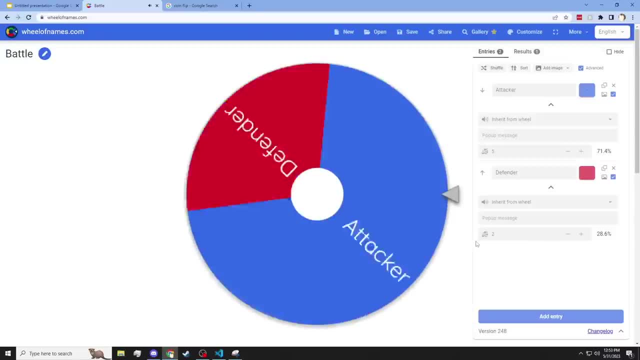 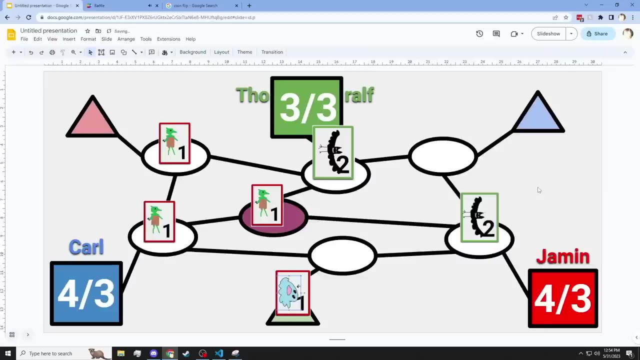 The angel moves onto the bat. yeah, I've lost worse before. Oh no, Oh no. How does that even happen? The movie of this, The movie of this battle, would be terrible. I'm enjoying this. No, no, no, no. 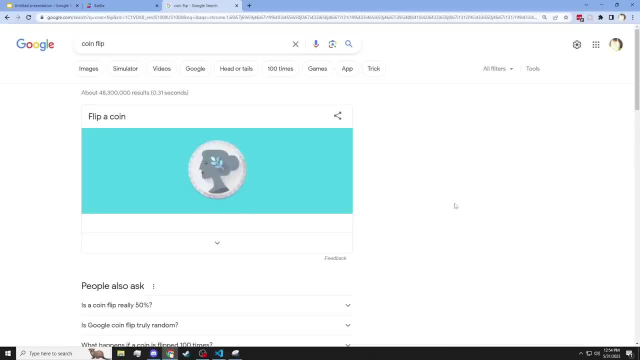 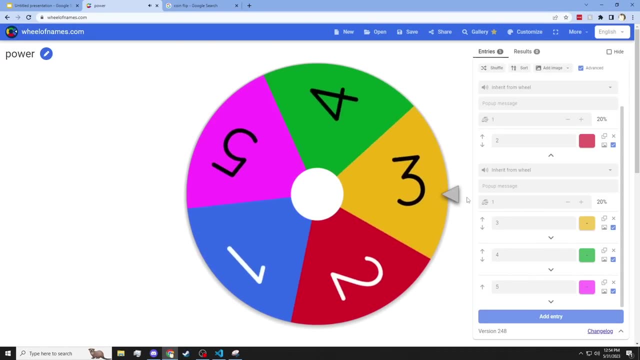 That's Jaemin's turn, Carl Heads. Okay, all right. all right, Let's make it big. I've got a lot of goblins to fight. I will settle for a four. I'm going to take the guy who's. 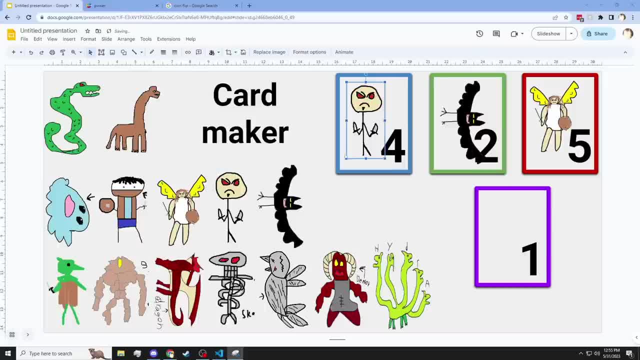 probably got a lot of bread to butter because he has two knives And his eyes are so red because they're tomatoes. No, he cuts onions. Does he use his eyes for the sandwich? What is this? Yeah, he's sad because he's crying. 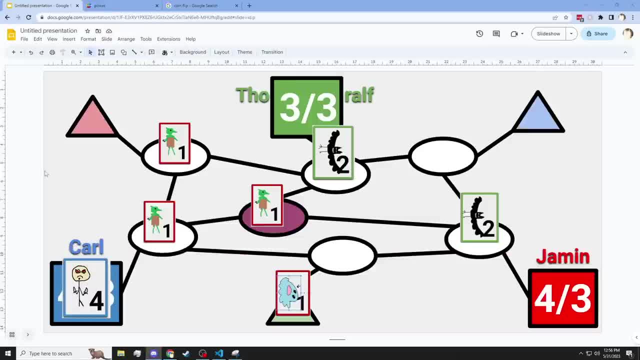 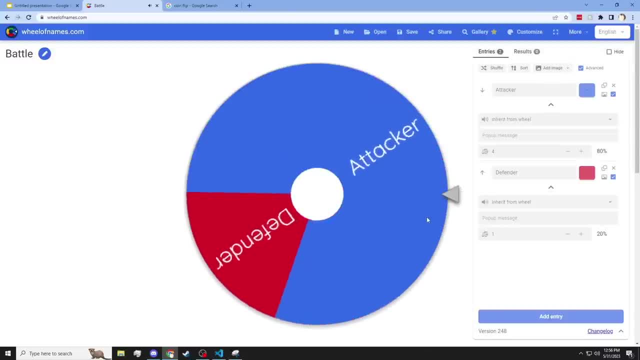 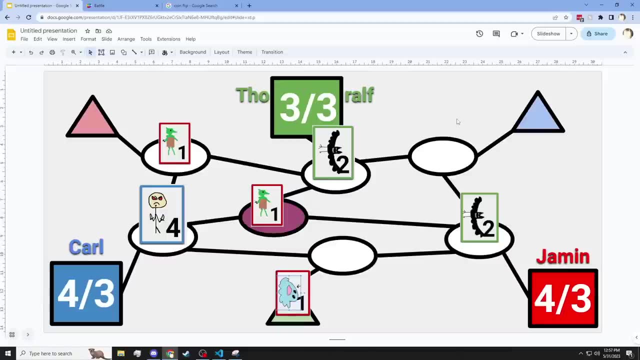 because the onions were his friends. Such interesting lore. Sid is going to move onto a goblin. The whale says: no Lips to butter. another bread Toffle. you're up. I kind of feel like my. We're going to try. 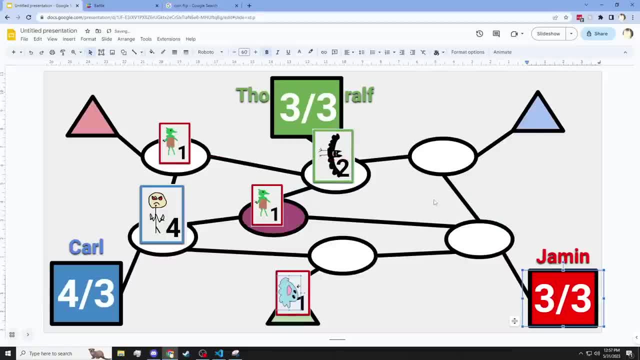 Okay, the right bat flies into Jaemin. Jaemin will take one damage and then you get to create a goblin. I'll create it on Jaemin. You can't create it there. It starts at your place. That's metagaming it a little bit too much. 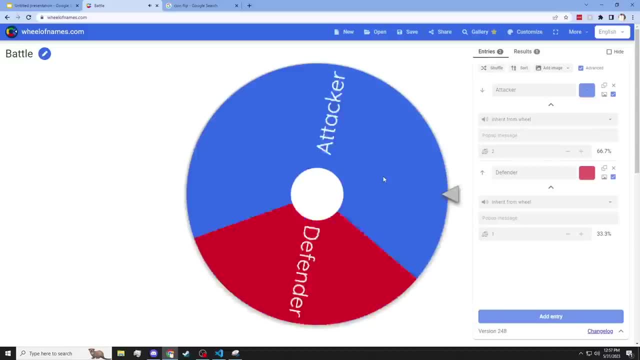 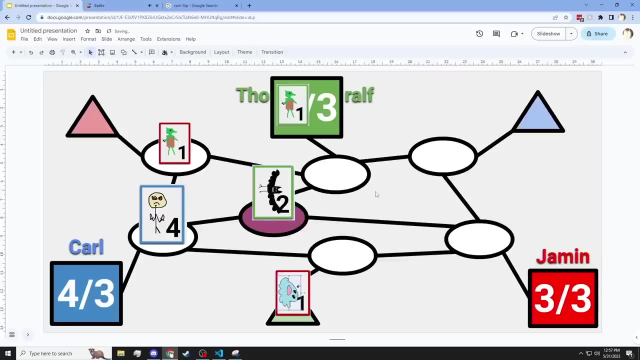 And then my bat goes into the middle. Ah, good, good, good, good good. They don't call him the goblin Sleisla for nothing. Sleisla, Sleisla, Jaemin, you're up Heads. 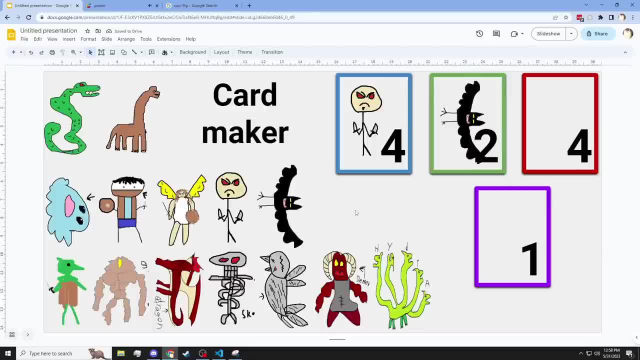 Perfect Core power is obviously the cat. That's a wolf. It's beautiful, Noah. Okay, thank you, Jaemin. I feel like you make the strongest creatures, but they always die. Yeah, that's how I feel too. 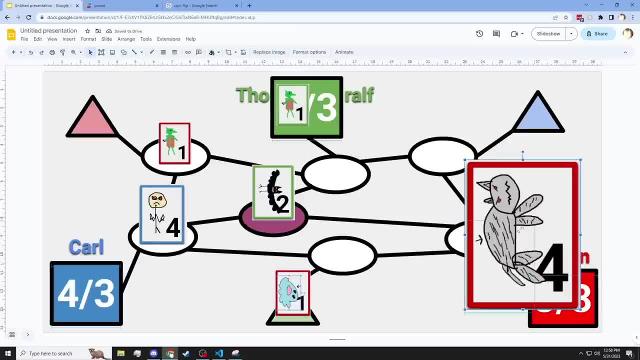 I also overwhelm the board all the time and they just all die all the time. Wasn't this board like Jaemin's city just two turns ago? Oh, that's happened like twice this game. yeah, I combine my abilities very poorly. 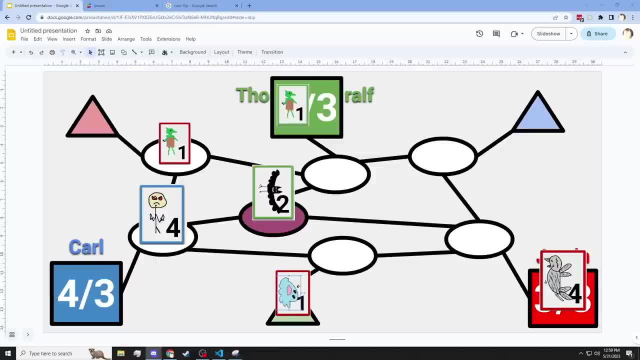 Anyways, Huh, yeah, Even Noah's like: yeah, that's pretty bad. Just let me know when that one comes up. I will. It's going to be awesome. My goblin moves onto my triangle. Karl, you're up, I would like to make a creature please. 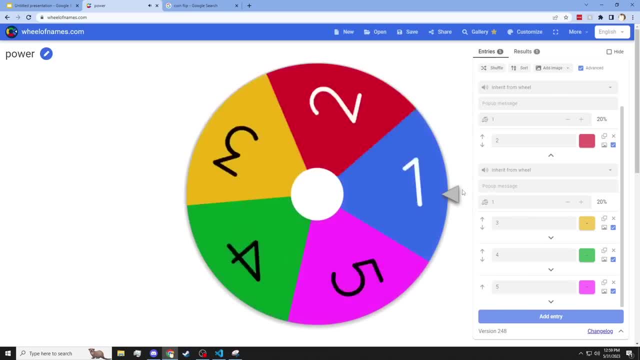 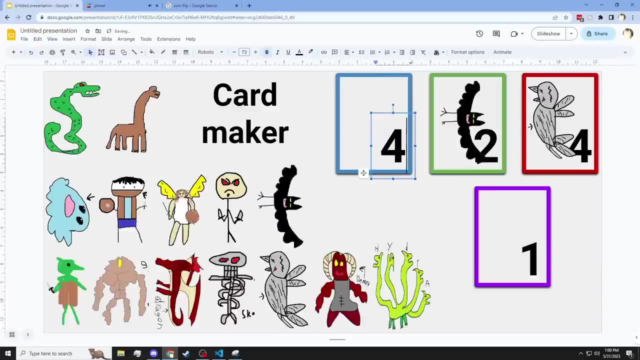 Heads. Oh yeah, Oh yes. Core power, This calls for a good creature. I want to have the uneven snake, please. What do you mean uneven? Well, look at it, it's just not even. 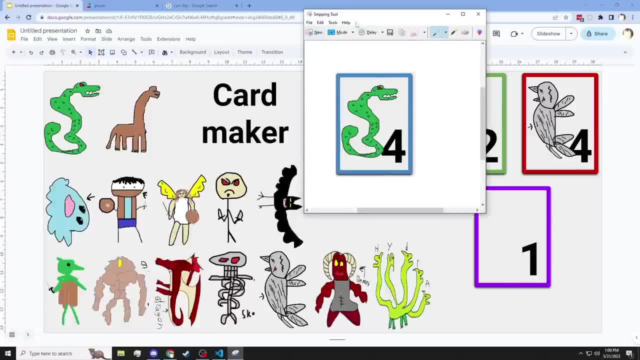 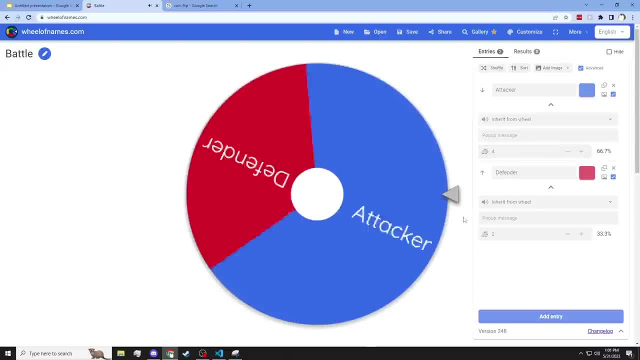 Sometimes it's really thin, sometimes it's really large. He's thick with three Cs. Time for the Batboy. My butter knives are coming. Come on Slicy. You call your bats Slicy when my guy It has two knives. 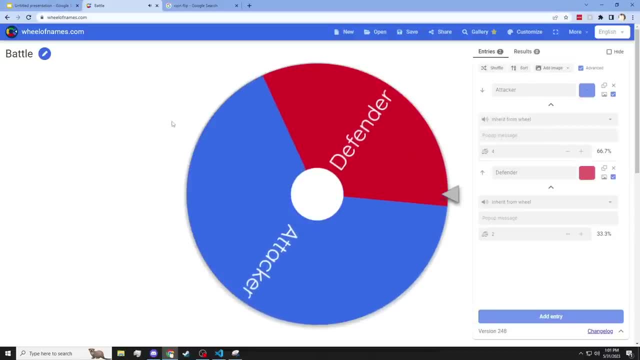 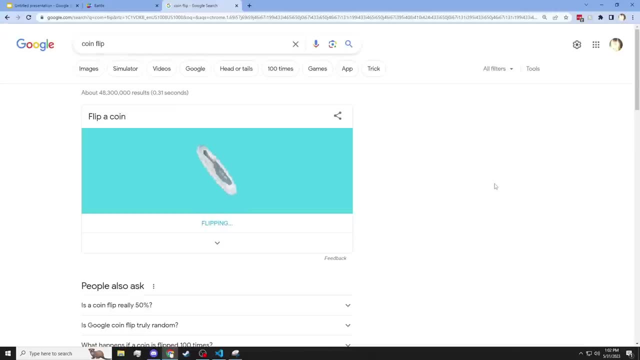 Slicey Woo, Oh, no Woo, Aye, aye, aye. That battered a hero, All right. well, the uneven snake is gonna move forward. Toffle, you're up. I would like to spin the good wheel. 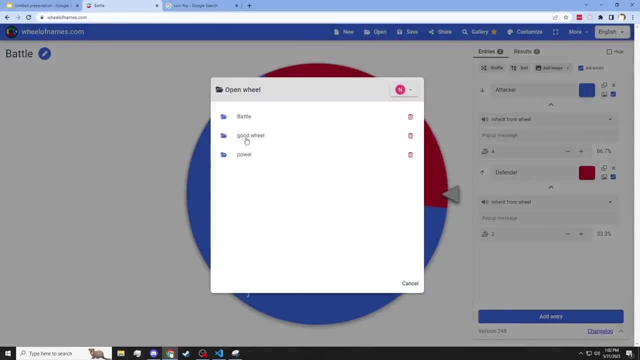 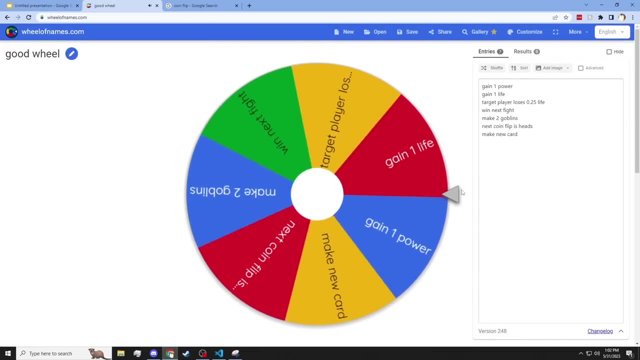 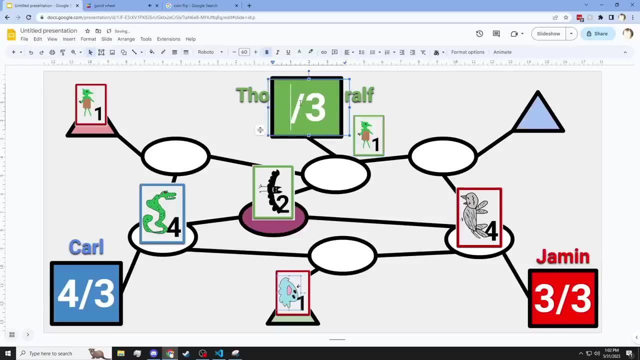 Oh yeah, you make a creature And make a creature. Oh, This is gonna last forever. Game over lice. Can I bargain into somebody losing a life? Yeah, who do you want to lose life? Kyle, it's gone. 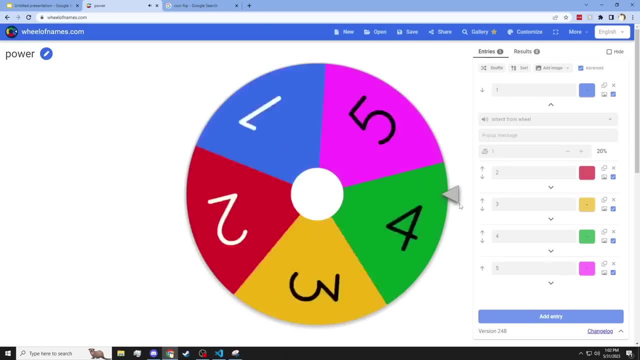 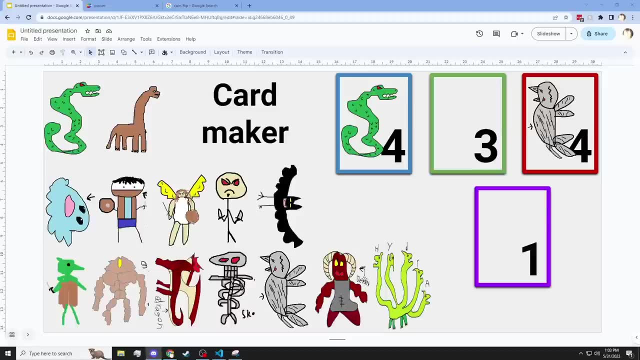 Oh, and then you make a creature: Uh-huh, Three power, And that must be the demon. I think, Okay, yeah, that makes sense, Okay, so it has come to my attention that I need to change the rules here. 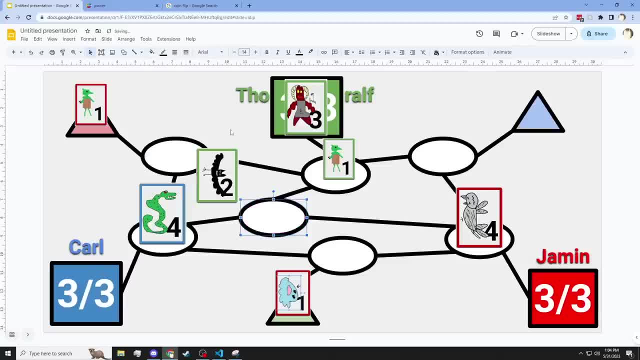 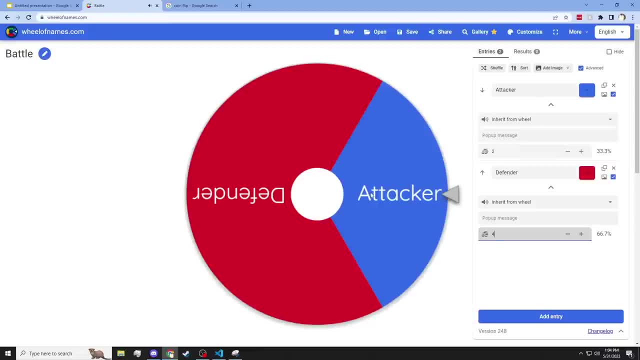 Otherwise we will be here forever. I'm going to make this space no longer a good space. Okay, Oh, okay, Toffle, you may now move your pieces. My bat is going to hit the cat on the right, I'm not afraid. 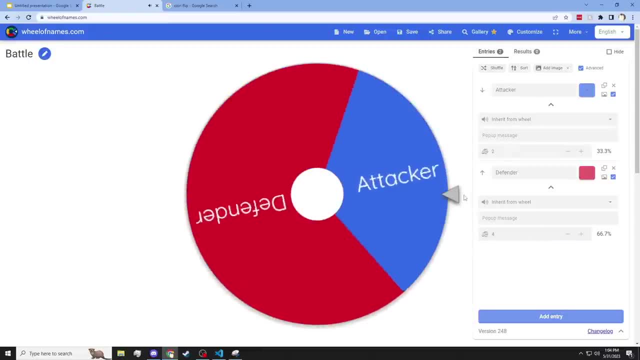 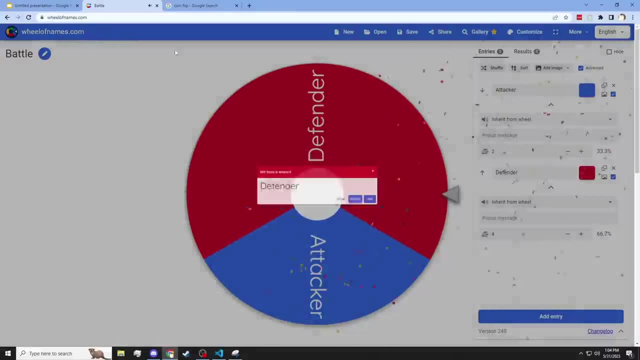 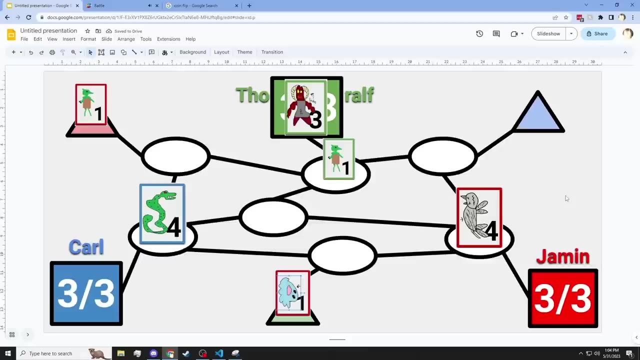 Zero percent Toffle Zero, Yeah. do you see this? Yeah, I mean, it's terrible at math Ding. Oh no, did one of my non-goblin creatures just die? Oh, you sound like a super villain. 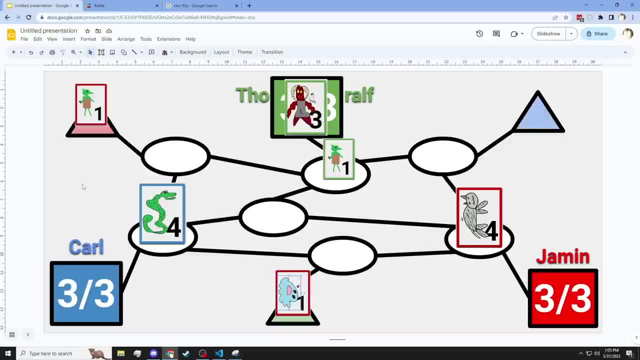 Then target player loses 0.25 life. That's actually buffed to one. Oh, Oh, What? So now we have to get rid of that Toffle creature, Jamin bye. Wait, so which creature? That's the demon that did this? 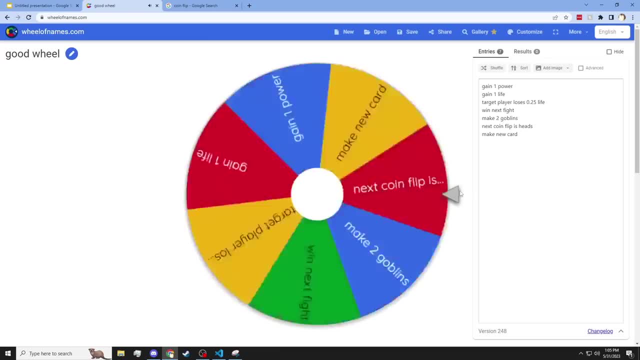 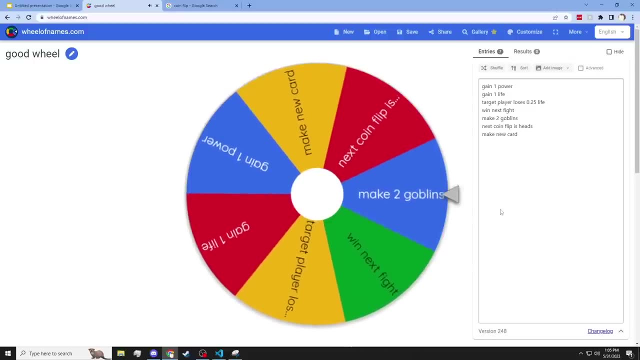 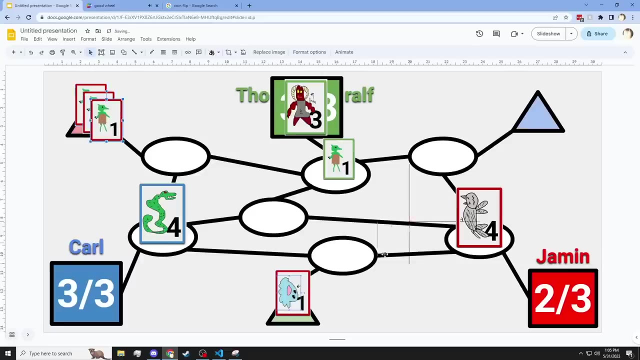 Maybe Jamin, you're up First. I get to spin the good wheel. Make two guys Nice. Oh wow, it is the good wheel. I loved it. Every time the clapping comes in, someone very enthusiastically cheers in the background. 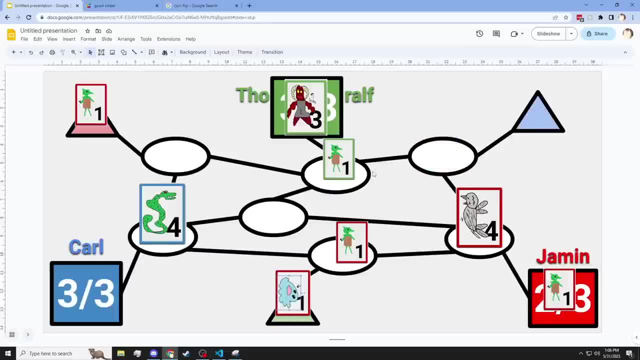 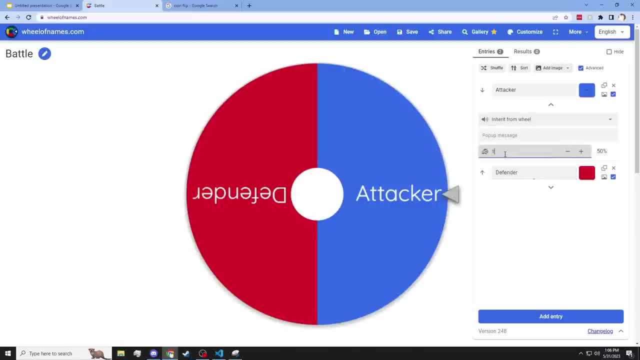 Woo, I love two goblins Tails. I guess the cat will move into the middle, the goblin will move out of my base and then the other goblin will fight the uneven snake. They're both green, but mine is a lot larger and less even. 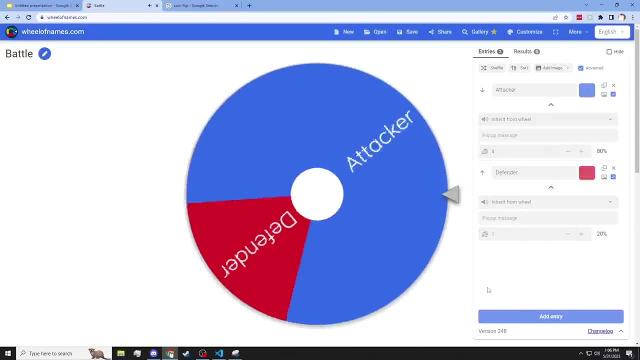 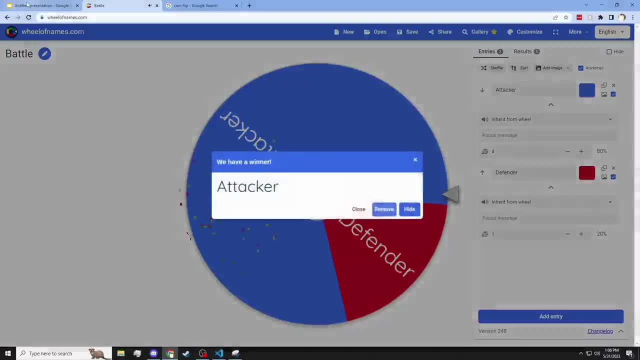 It's not looking good for you. Oh wait, no, this is reversed Attacker. is the defender? All right, Easy, No, Yay, Well, this has been an even six. That was a good one. That was a good one. 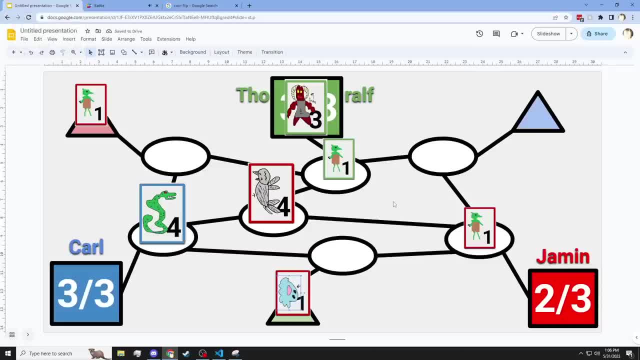 What do you expect? Basic biology, Jamin. That was my turn. Carl, you're up? Nope, I can't even swear, because Jamin gets a goblin. I would like to move the uneven snake. So if that big snake hits Jamin, it still just does one point of damage. 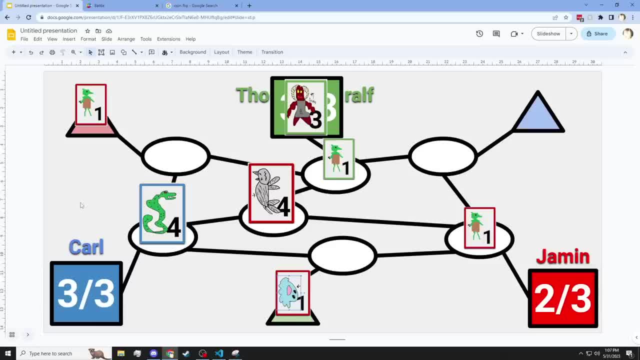 You know what? We'll buff it to say: I'm going to change the rules, just because this has gone on long enough. The amount of damage that a car deals is equal to its power. Whoa Jamin, here I come. In the world of Noah, there are no rules. 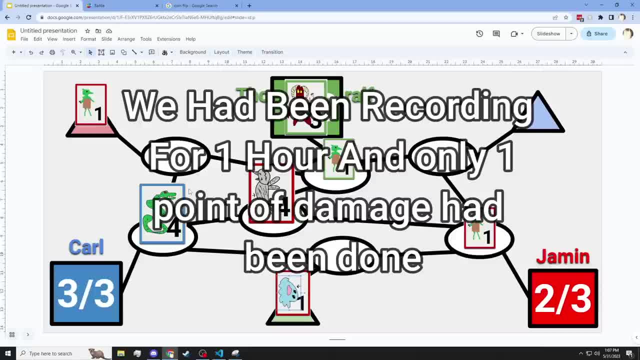 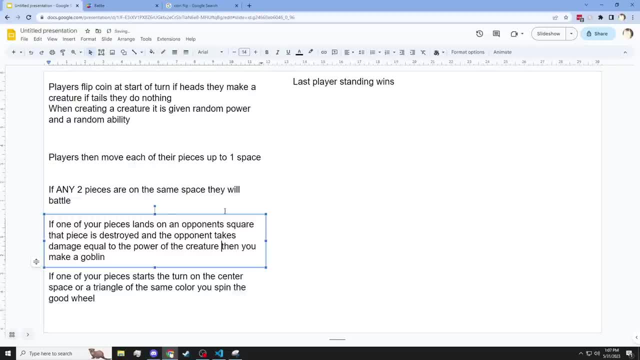 I think it's a good idea. It's one of the things in the game where when a car deals, it's equal to its power. Whoa Jamin, here I come. In the world of Noah, there are no rules. 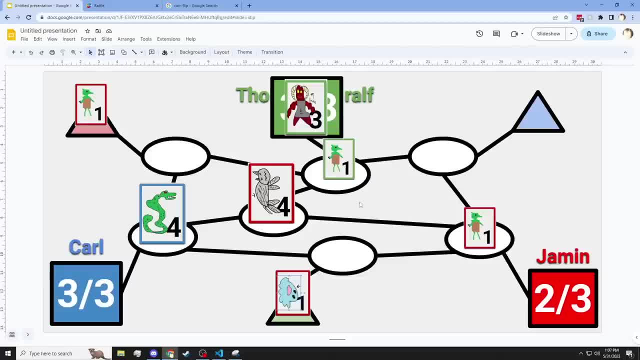 Exactly, It's Noah Cannon. I would like to move the uneven snake towards Jamin. It's a coming, And you know what We're also going to say. Well, we'll just say: the creature also doesn't die. Whoa. 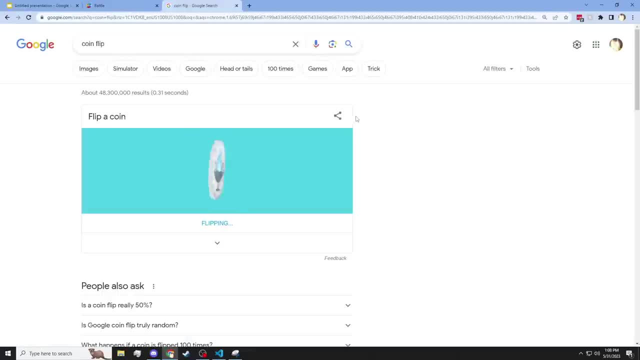 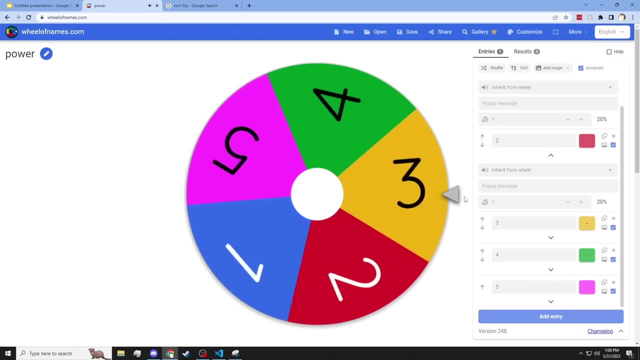 Okay, Tafel, you're up. Nice, Someone's calling on you. It's Tafel. What, Wait, what was that? I don't have anything. It's Tafel. Okay, Tafel, you're up. 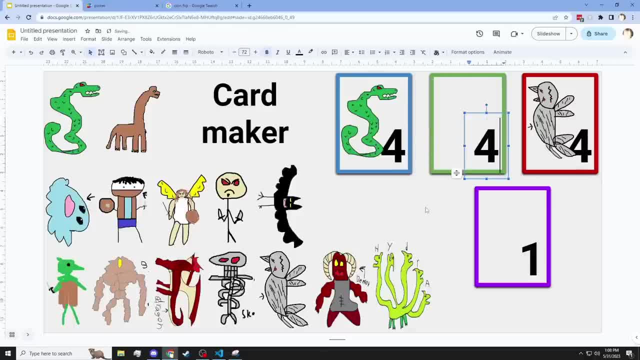 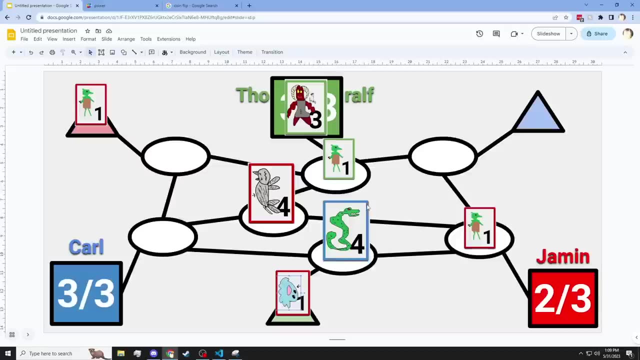 I love that all of Toffold's creatures are not just like instantly lethal to all players. If I lose, I have a spam button. If I just swear like a hundred times, we all lose. When this enters the battlefield, move opponent's card to any circle. 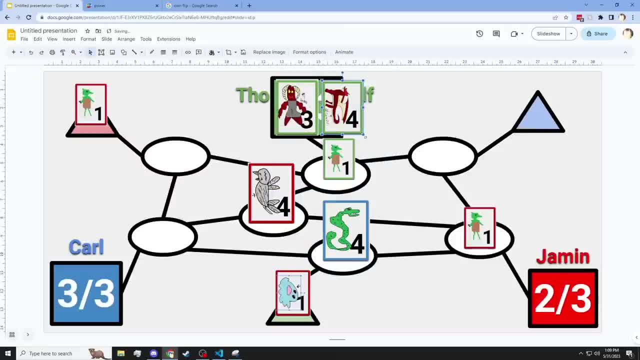 So I can take any card and move it to any circle- Yes, An empty circle, or a circle with a goblin or a wolf. This does push these cards out like this. Hey, Can the demon and the dragon switch places in moving? 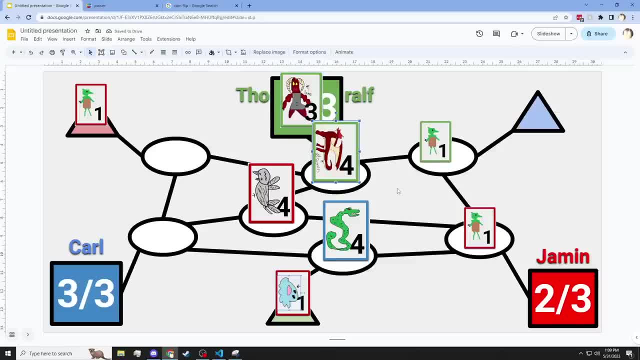 Sure, why not Nice? All right, I'll move Jamin's goodwill goblin in front of Carl's house, And then the dragon moves left to Carl And that's it. Okay, Wait, they already did. They switched places in moving. 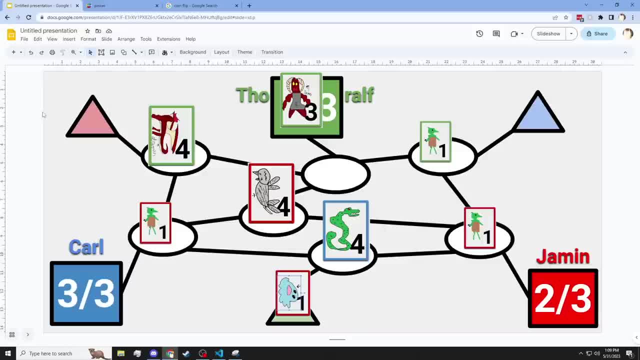 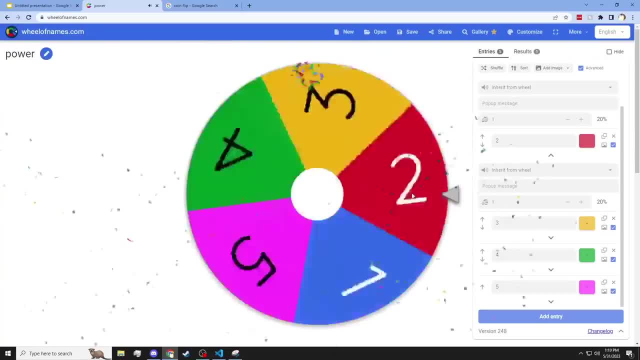 Yeah, You can't have the dragon be pushed out. No, I said that it was okay. Jamin, you're up Heads. You get to make it All right. You guys are so many creatures. Cool Man, I love the cheering. 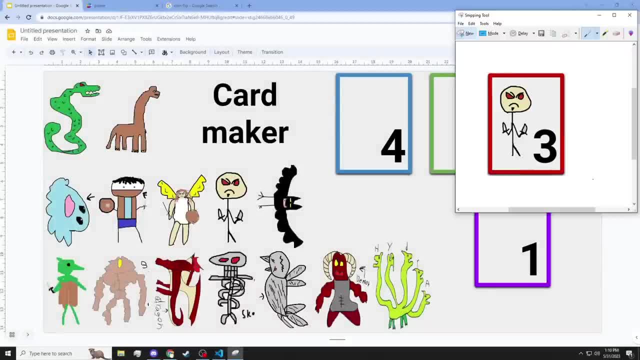 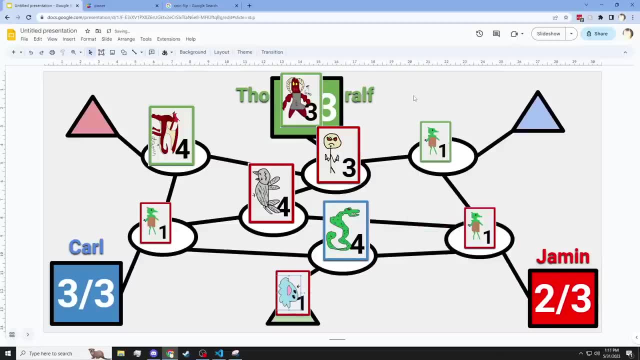 Three power. I'll pick the bandit. When this enters the battlefield, it teleports to any circle in front of Tafel's house. Oh wait, Does it move now? I hope it does. Yeah, it's your turn. 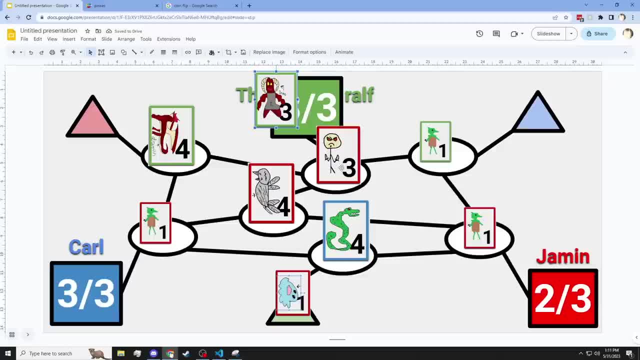 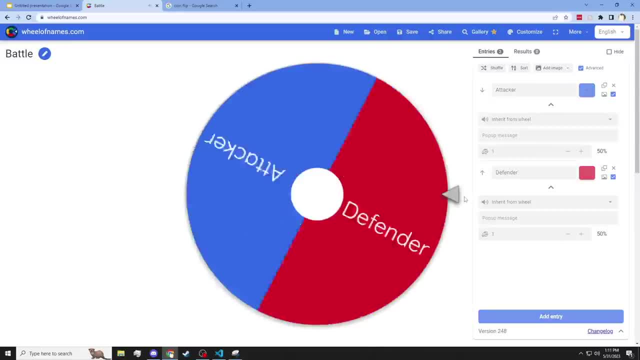 You can move your pieces. I'll move my bandit onto Tafel. Wait, does a coin flip to lose the game? Oh God, Here it goes. If Tafel's monster dies here, so does Tafel. 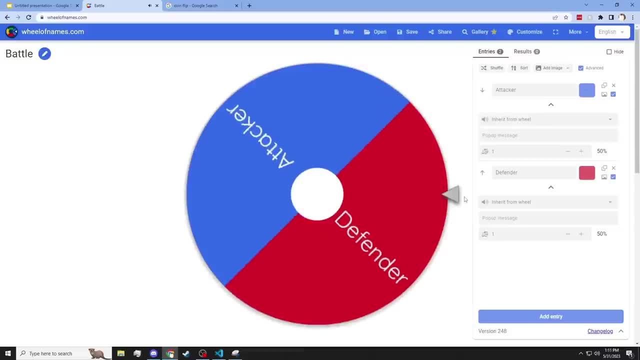 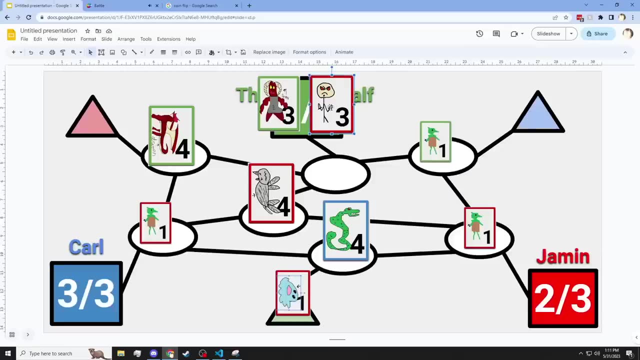 Or does Jamin have to attack it next, Next turn? No, no, I just go attacks. No, no, Yeah, No, no, no, Yes, yes, yes, Yeah. The defender wins. It was a good try. 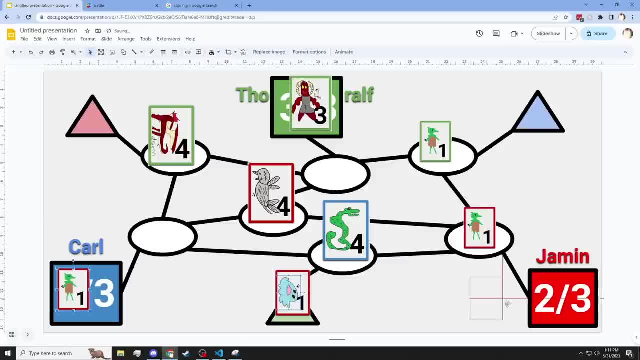 All right, My goblin goes, Carl. This goes back to your base and Carl loses one health. And then my cat goes towards Tafel, Your cat Wolf. of course Wolf, It's got an arrow on its back, Jamin. 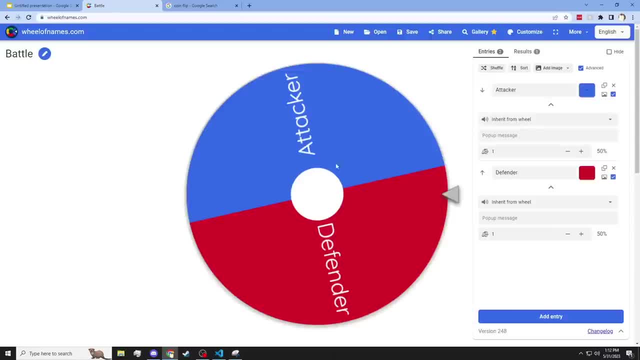 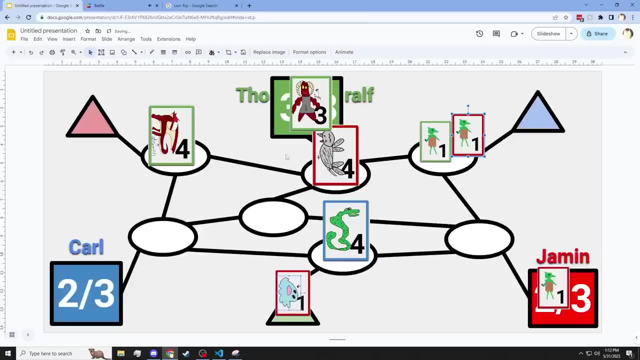 And then my goblin attacks Tafel's goblin. Actually that seems stupid, But then again Whale's already spinning. It was stupid. Okay, Carl, you're up. Okay. first I'd like to make a creature. 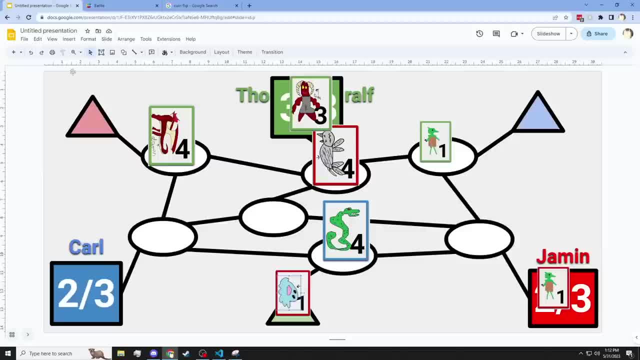 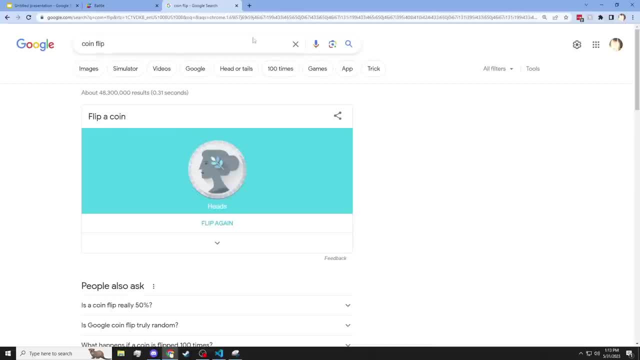 Wouldn't it be awesome if I rolled a one and I made a goblin and I give it some cool abilities and I got tails. I will move my uneven snake towards Jamin Tafel. you're up Heads. Please give me five. 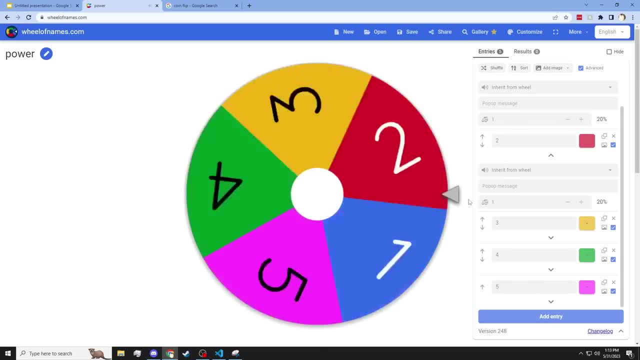 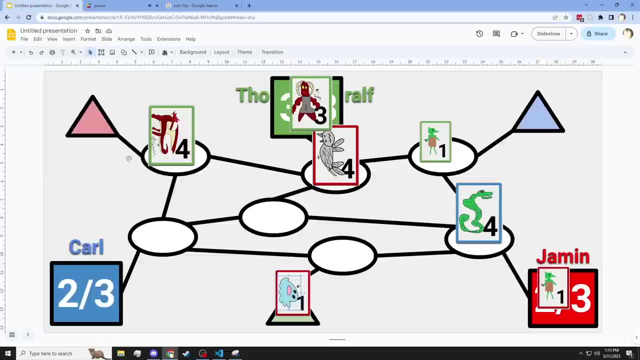 Must be nice to win a coin flip. Huh, Any five. I'll take any five One time. Every time we've asked for a five, we've gotten a one. I have an idea. I would like to have the slime. 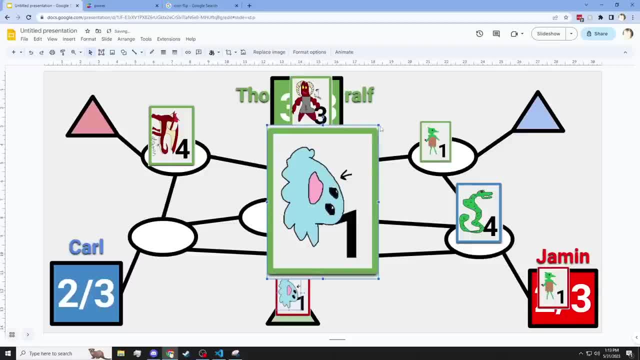 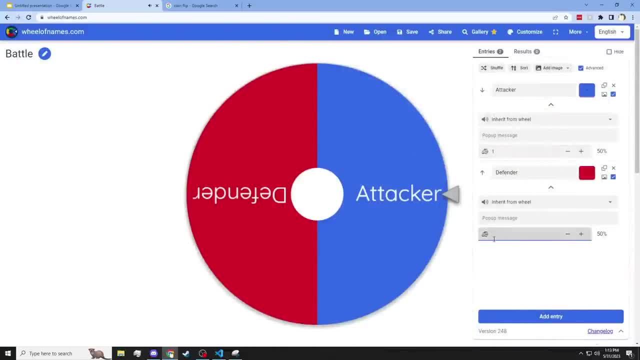 All right, And then my slime is going to attack the wolf. I really hope it doesn't die. The sarcasm is palpable. I don't know what I said. Is this your turn to pick the last card? I don't know. 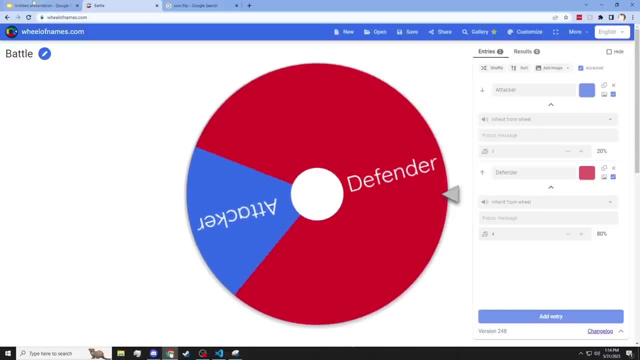 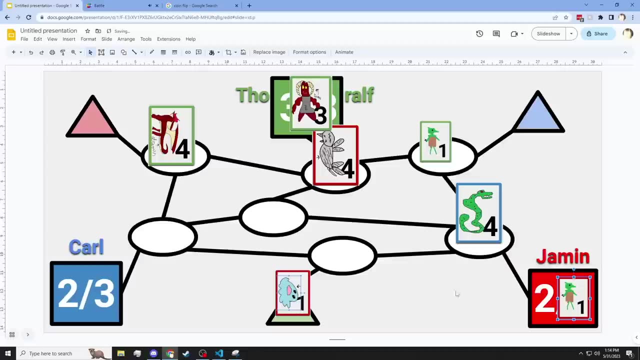 I'm gonna do what I said on um Good, Ah, Shatang Strudels, I would count that as a swear word. Then I would like Jamin to lose a life. Okay, Then my dragon attacks the wolf. 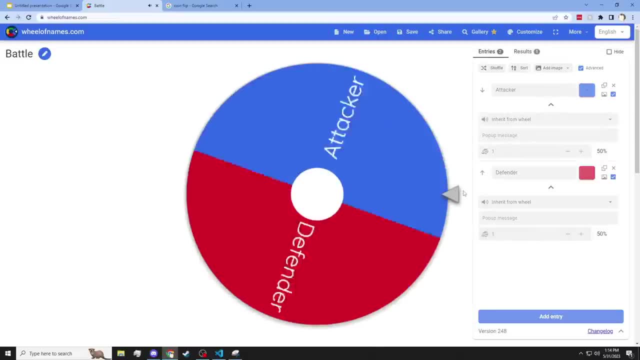 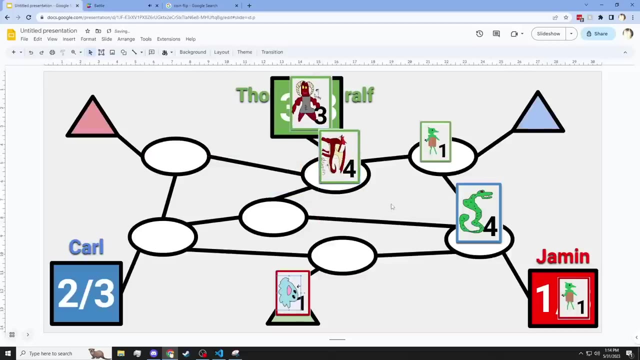 I really hope I'm winning. I feel like this is lethal to me. It's not. Ooh Wait, Kyle, you're not. you know You're not effective. yeah, but if my- um, so my cat- had a secret ability, yeah, it gains one power, okay. 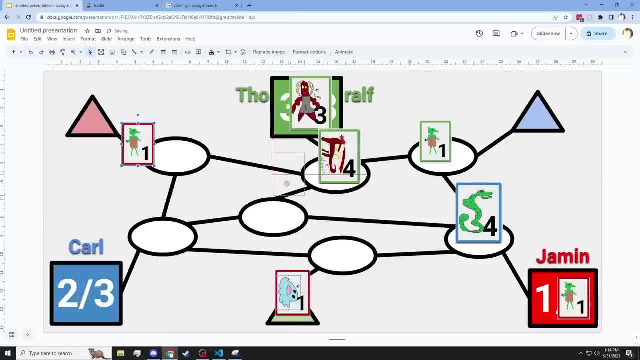 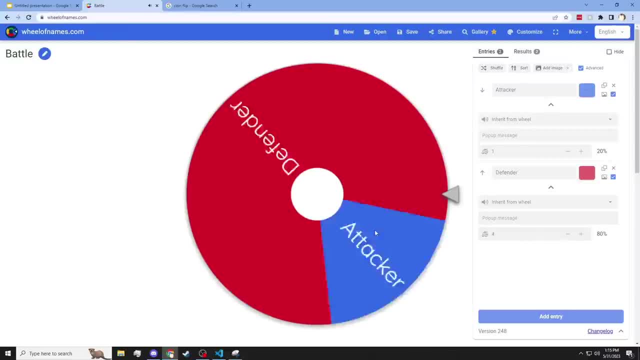 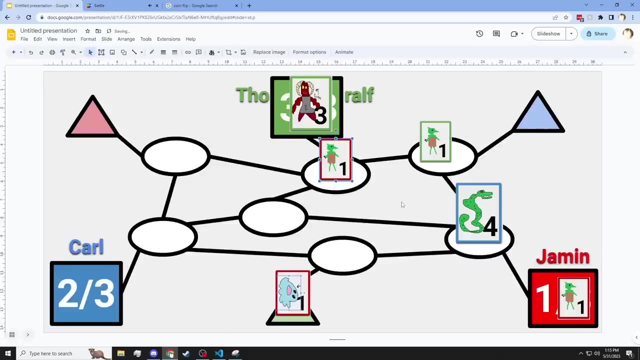 it's gonna come back as a one power goblin, uh, and then it's gonna fight the dragon again. nice, no, not nice. you can say a bunch of bad words and but then you win, but you're dying anyways, maybe bleep. actually, how does this, the stack, work? oh no, i don't know. i just wanted to make a bleep goblin. 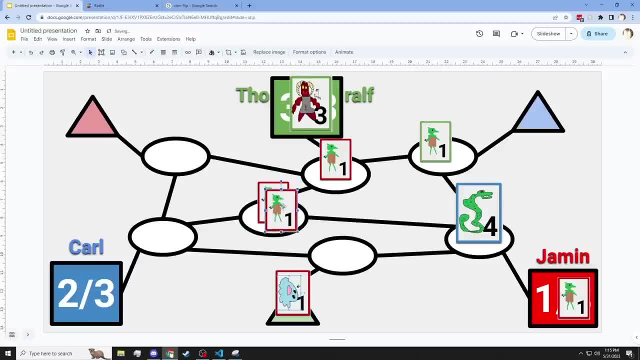 oh, there's another one. he said: bleep goblin. that's another token. yeah, but if what happens when the space runs out? i don't know. they just all overflow to everyone. but wait, if yamin is dying on the stack and i make infinite goblins making tarp and i lose the game, then is it a draw, you don't? 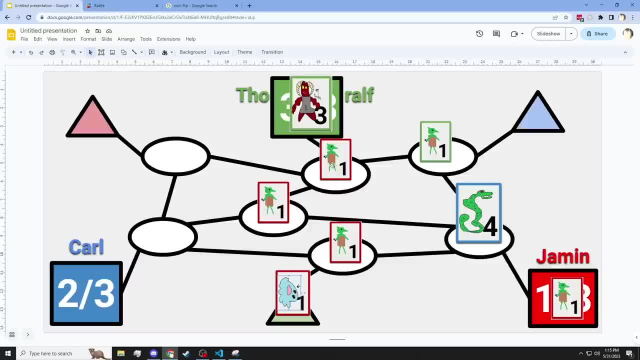 know what happens when somebody dies. how well, i want to find out. but it's only jayman's goblins and they all go away. yeah, but they kill us first and then he dies on the nah. we're not doing that, we're not making. he's dying. no copy or paste that much. he's dying, he's dead already. are you choosing? 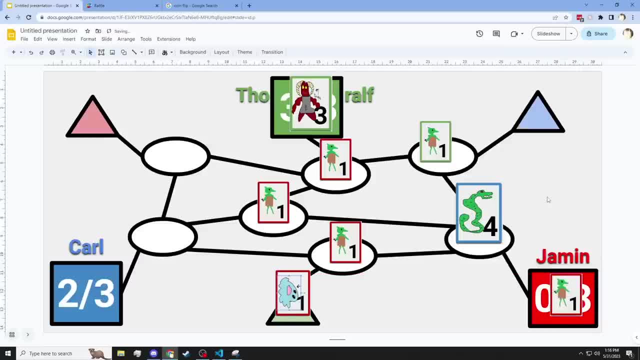 what damage, jayman? yes, of course. so, jayman. you may be dead, but you can still move around your remaining creatures. no, yeah, i'm not making goblins. i regret the two swear words already. um, carl, i swear allegiance to you. uh, yamin, bleep, bleep, bleep, bleep, bleep, no, no, no, no, no, no, wait, wait, this is so. 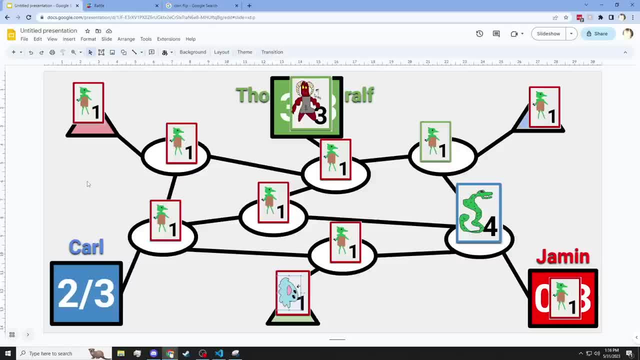 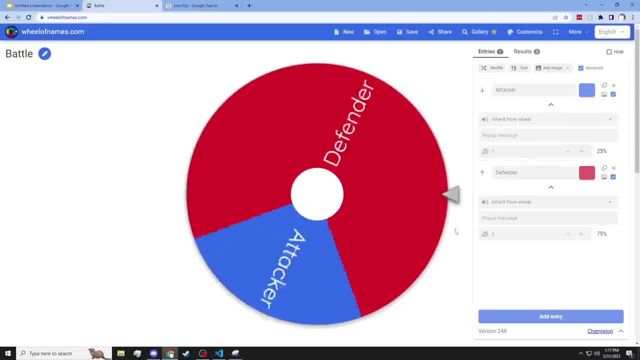 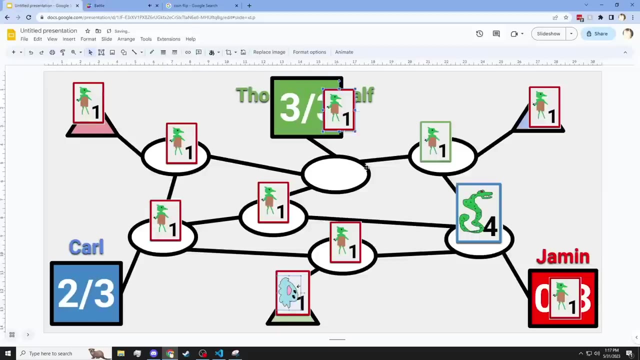 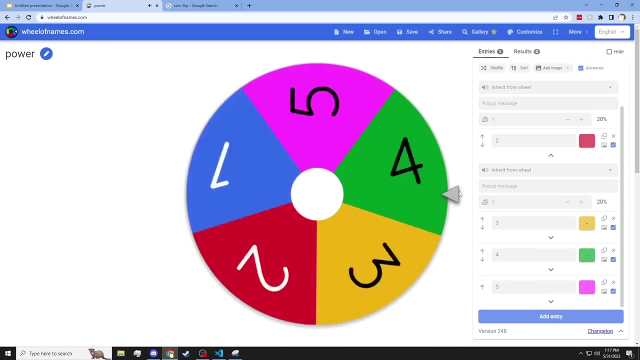 satisfying. there are now no more spaces for goblins to go. uh, jayman, it's your turn. my goblin moves on to topple the demon. oh god, this feels like an uproar. he'll battle out. yes, yes, attacker is one. carl, you're up, you get a creature. i want a four. you want a four? well, 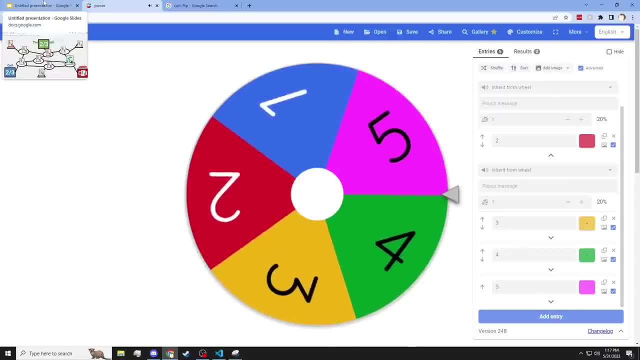 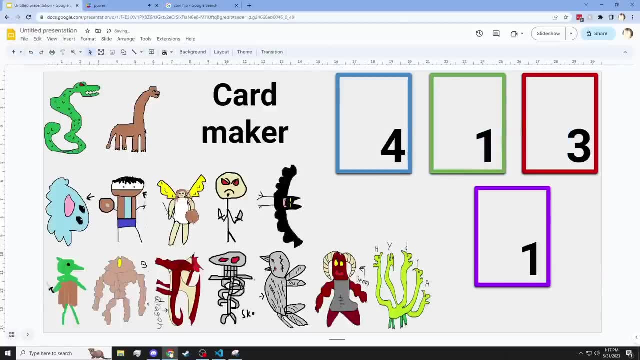 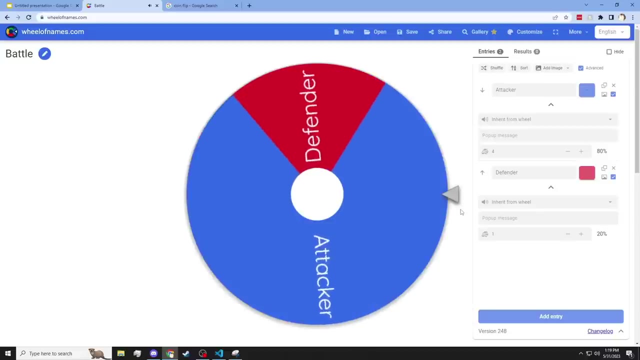 uh see, all right, you can get a four to. oh, that's crazy. oh see, every time you have to reply, you gotta one. i i met a game bit. i would like, uh, the guy with the hot pants, i'm gonna come for todd's goblin. Oh no, no, that's not not gonna not going to win that one. yeah, i mean, i'll reply on you. 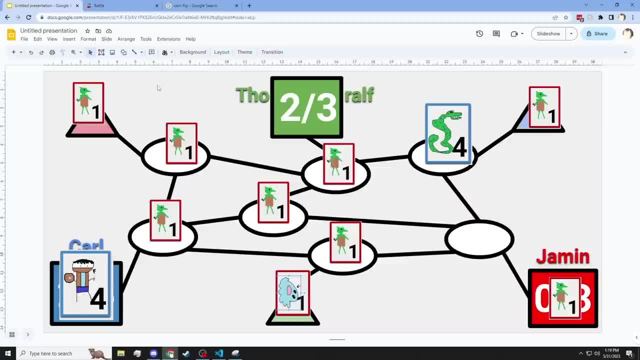 to make some space for my hot pants guy later on. sorry, my my military goblin operations. don't mind it, jayman, please let me hit kinkos bad. jayman, you're up for simplicity. can i combine all of my goblins into one mega goblin machine in? 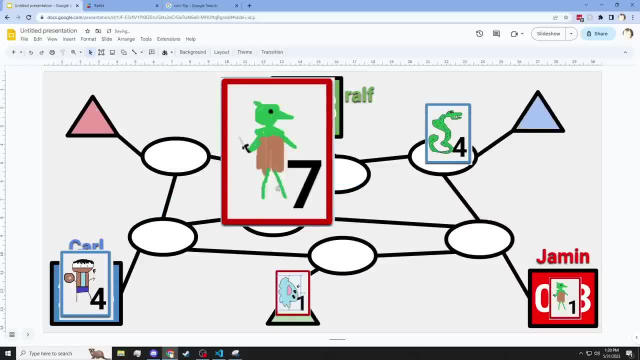 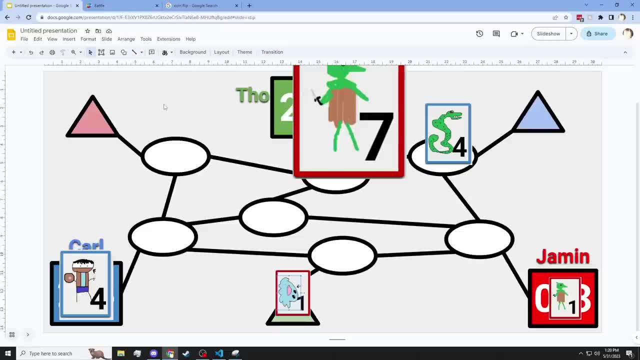 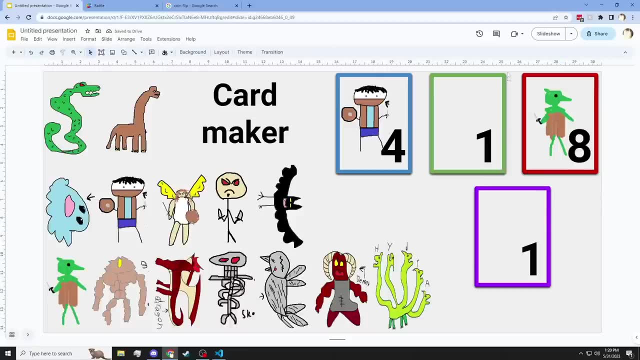 the middle of the board. oh no, all right, i'll move it one step towards toffle. it's a big ball. uh, carl, you're up. i'm afraid of moving the snakes closer, so i'm just gonna move the. uh, the guy with the blue pants. this is eight, eight. yeah, we forgot the goblin in my base. 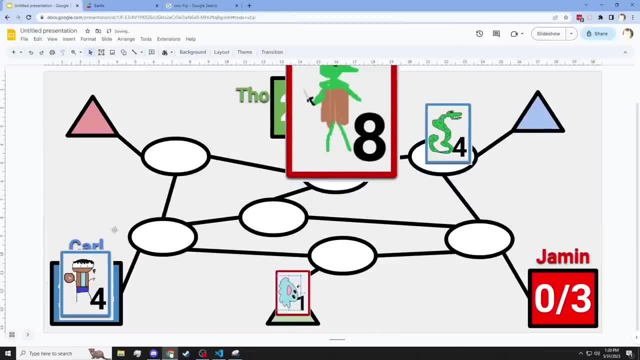 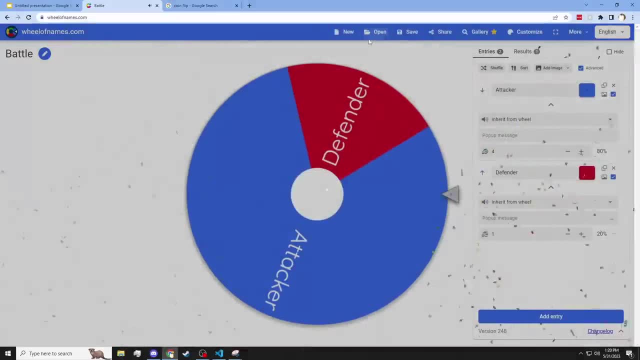 does it really matter? um, i would like it a bit bigger. the way the game go, it matters. yeah, yeah, uh, i, i would like to move the guy with the very short pants up one square closer. toffle, it's your turn. um, i would like to hit heads. it better be huge. 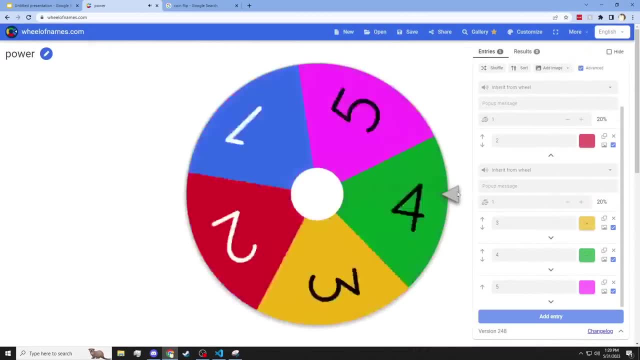 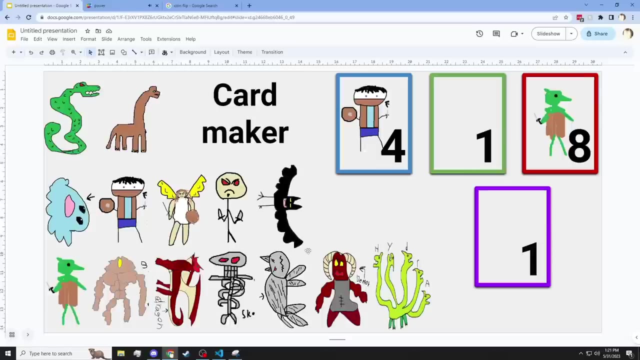 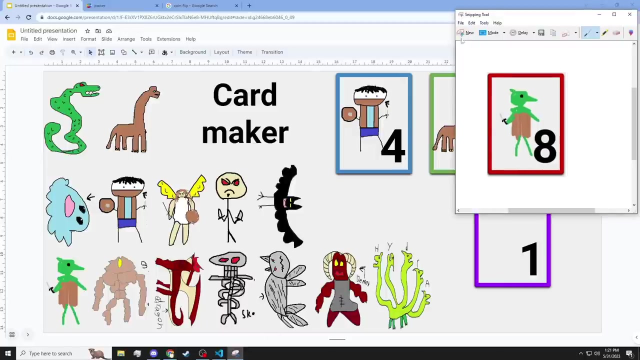 okay, yeah, all right, that's good, huge, huge. so when this creature enters the battlefield, destroy card with six or more power. no, you know on your list, i know, i know how toffle sounds when he makes stuff up. okay, i have 12 and four left. that is when, when you had one or less life at the start of your turn. 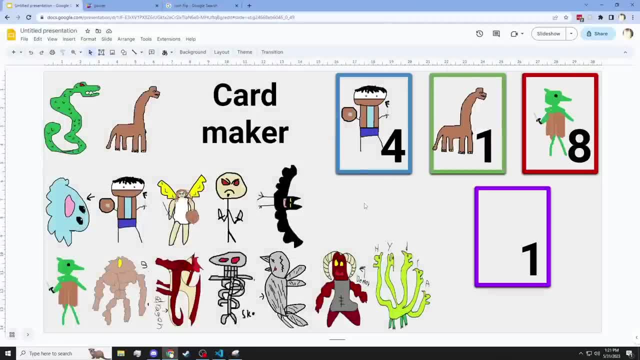 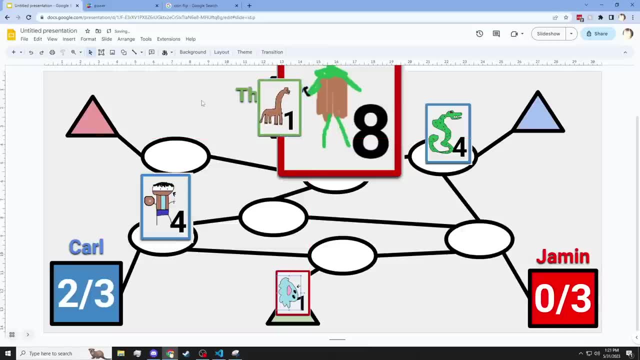 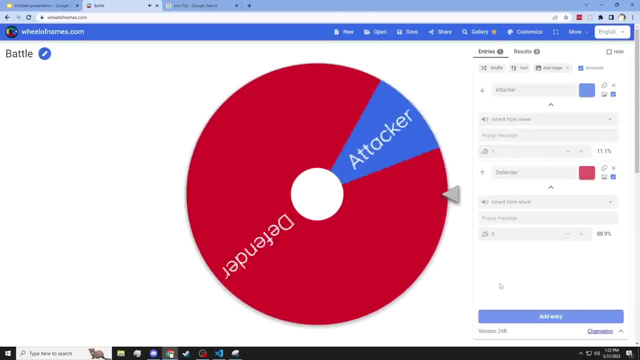 target card loses one power. no, i mean it could get through the goblin army at some point. all right, this is epic goliath versus david. i think it's poetic that it's a yamen charge. so yeah, attacker one power, defender eight. oh my goodness, attack is gonna win. 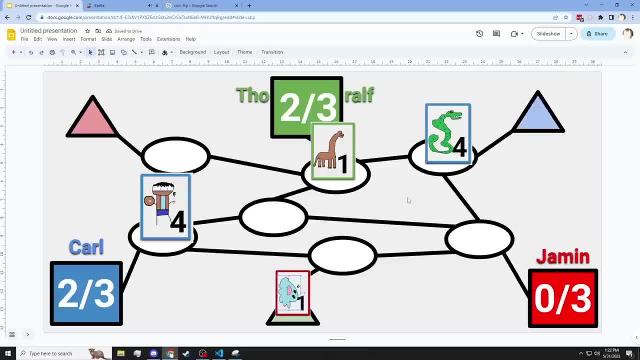 jamin, you're up. carl, would you like to swear? no, carl, no, oh wait, you still have that silly towel. bleep, bleep. i love how you can just summon goblins. it's a very, very fair mechanic. um, yeah, i'll leave it to the game if this is my turn or if i can move these. 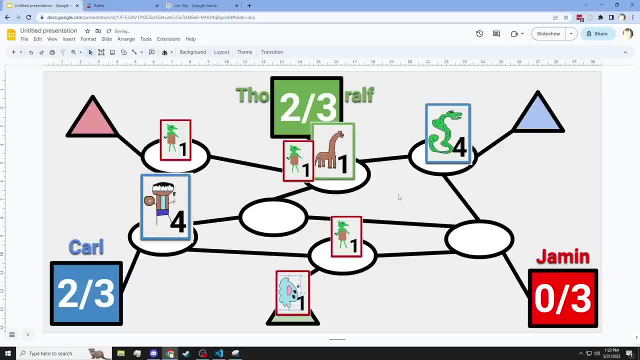 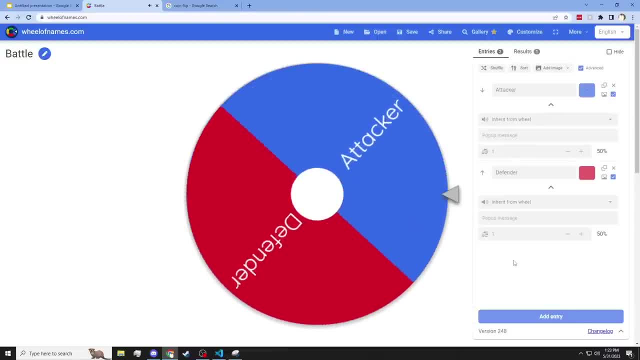 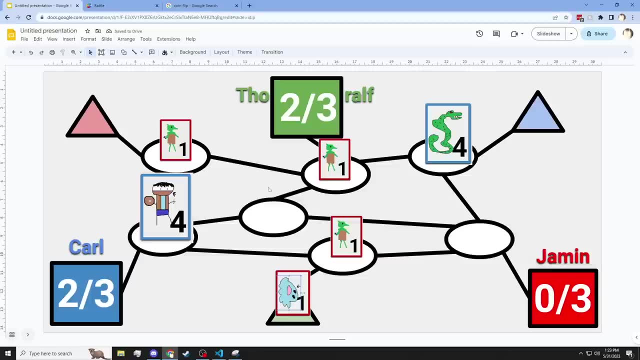 could you please move one of the goblins so i can move my guy with the short blue pants. all right, no, oh, ironic. ironic that eight goblins couldn't take down the long neck. It didn't bend down to the one. Carl, you're up. 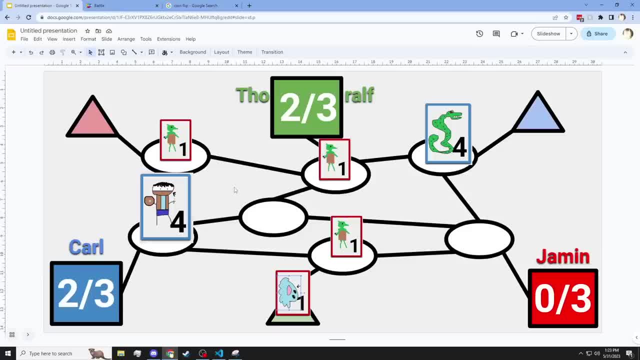 Tails. Okay, My uneven snake is going to go fight that goblin. Oh, that's Yemen's goblin. No, no, it's going to stay chilling. Oh, can they hang out in the same square without fighting? We'll say they can. 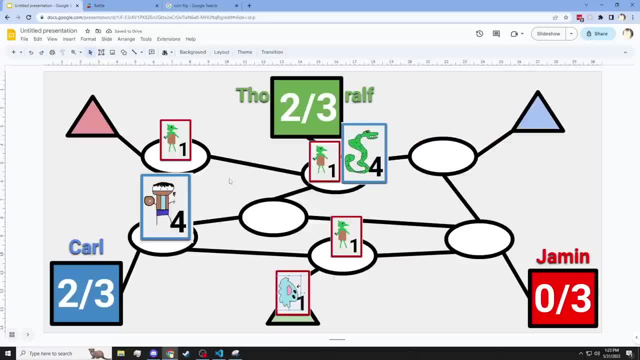 Oh, they're friends, They're both green. I would like the person with the tiny sword and the towel- blue towel- around his waist to go to the middle. It's a very long, slow death Tafel. I'm going to make you a deal. 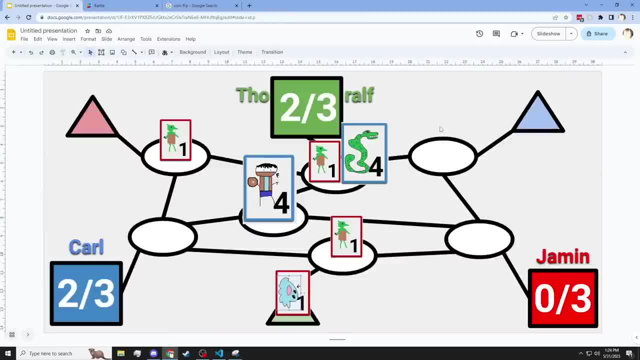 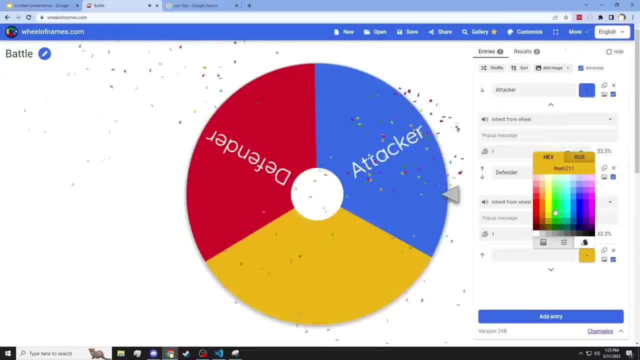 And you can choose to accept it or not. So for the rest of the game you make no more creatures, but I'll give you two creatures right up front. Hit me, Poop army, charge forward. Oh, what's happening? Okay, now we're going to have. 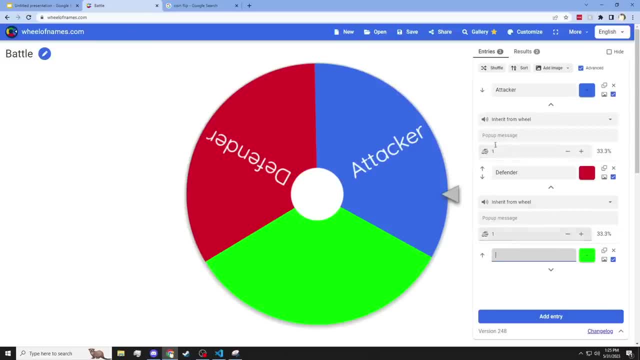 a three-way fight. Nice, Oh, that was what the fourth color was for. All along it was there. Not at all, was it? No, Listen, I just make this up as I go along. Did Noah just think that we'd have a friend with us? 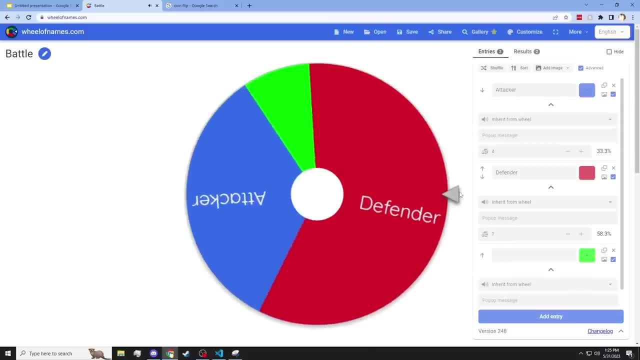 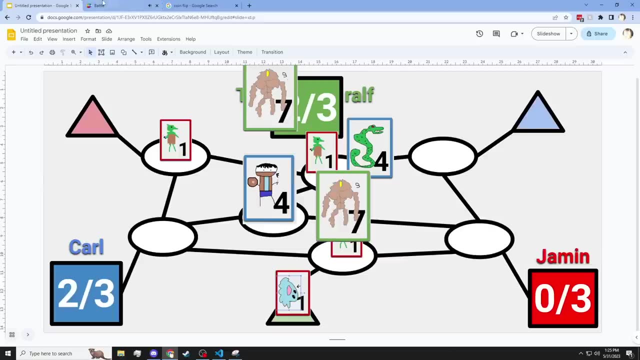 No, no, That was just in case I felt like it. Oh Wait, who's the defender? No, shouldn't I. That's just red. Oh wait, I should be the seven. Listen, This is all that matters, okay. 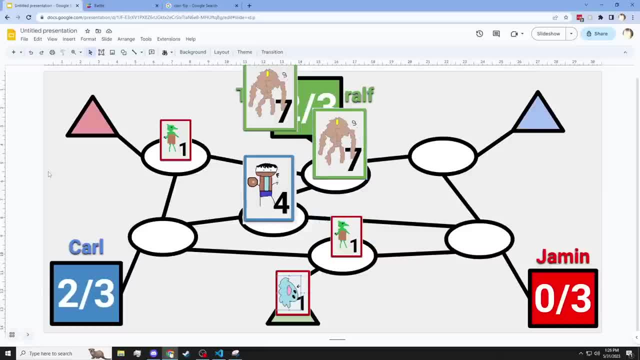 Yes, There we go. Justice, Yeah, yeah, yeah, Of course. So if my card loses a battle, it becomes a copy of a specific card I own. Okay, Wait, the goblin. No An even snake.